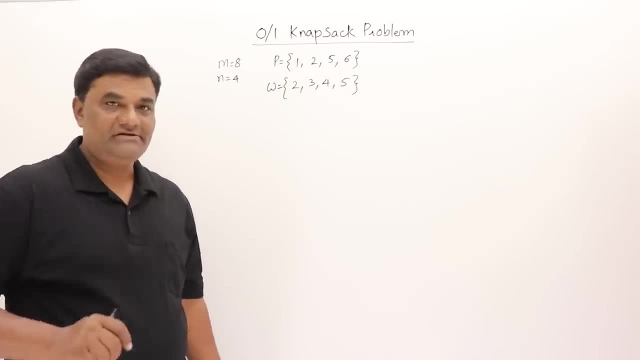 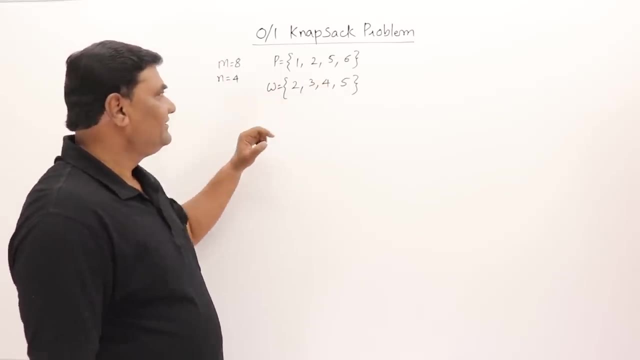 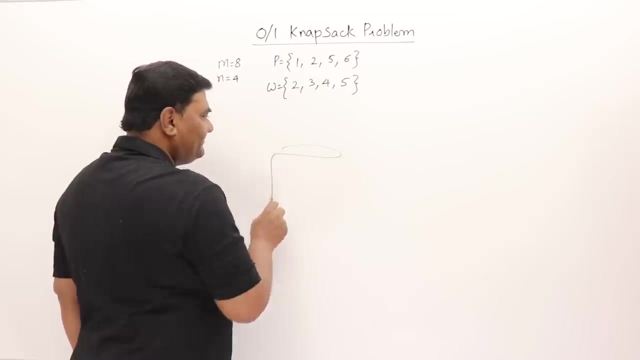 for solving this one. So there are two methods. We will see both the methods. First of all, let us understand what the problem is. Here I have some four objects. For each object there is some profit and there is some weight And there is a bag of capacity M, that is 8. 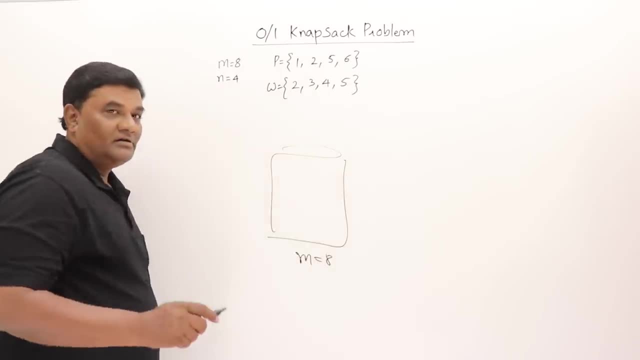 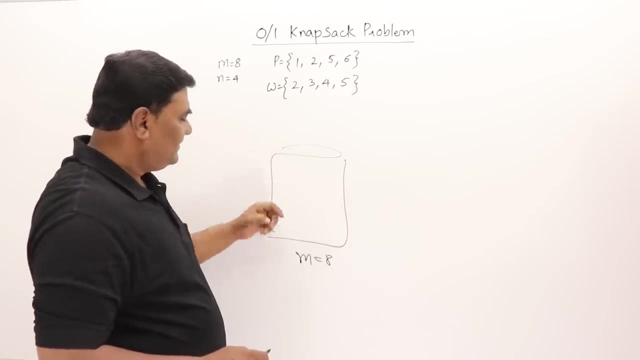 is given. The objective is to fill this bag with these objects, So can I put them all? See, the capacity A is 8, but the total weight of all these objects is 14.. So I will put them all in the bag. So I will put them all in the bag. So I will put them. 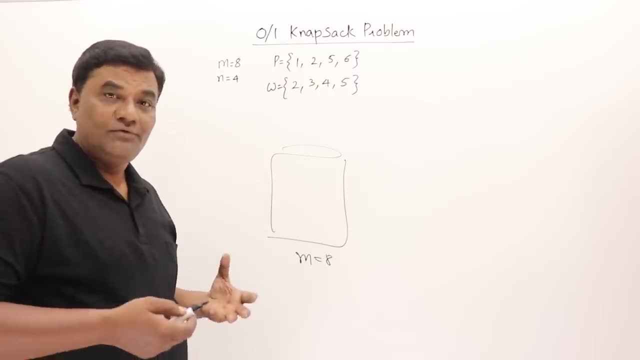 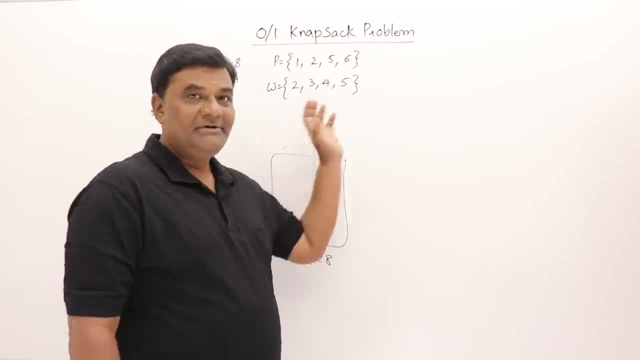 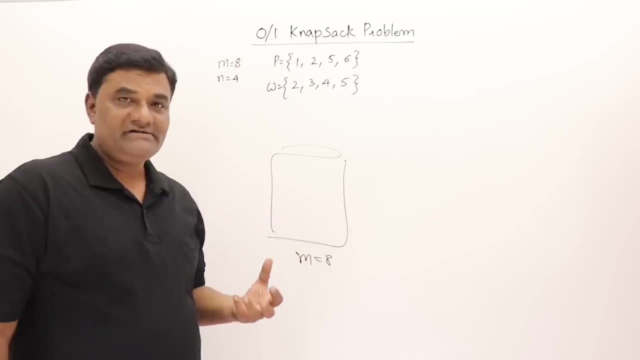 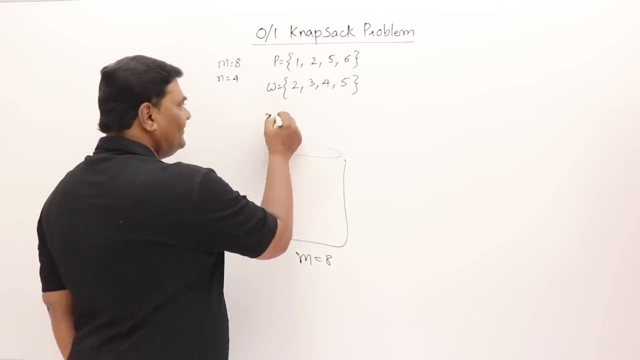 objects. There is subset of those objects And I have to carry them and sell them at other place. So once I sell I get this profit. So I have to fill the objects such that the total profit is maximized And I have to give the solution in the form of a set for each. 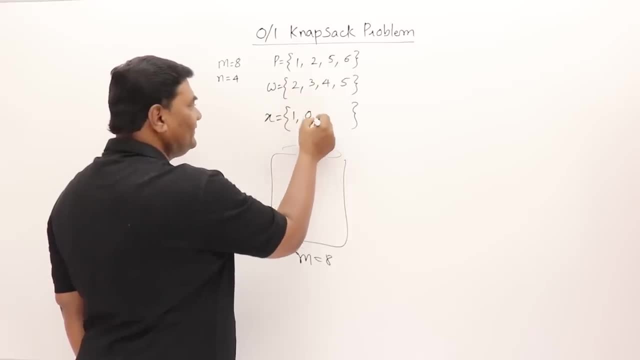 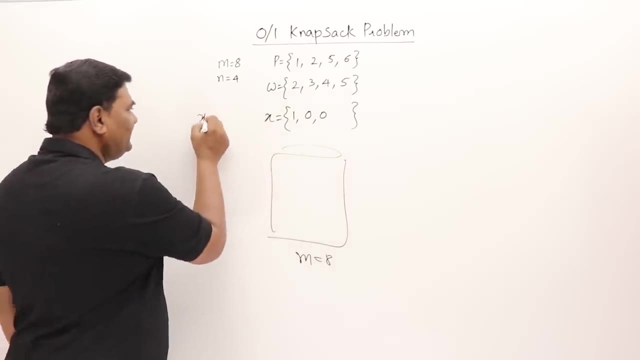 object Like, for example, this is included and this is not included or not included. Like this: I have to write down which one is included and not included. So it means I can write down each xi either 0 or 1.. Means the values can be 0 or 1, but not fraction. So it means 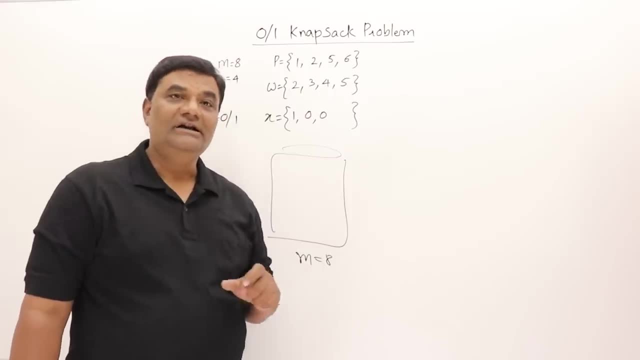 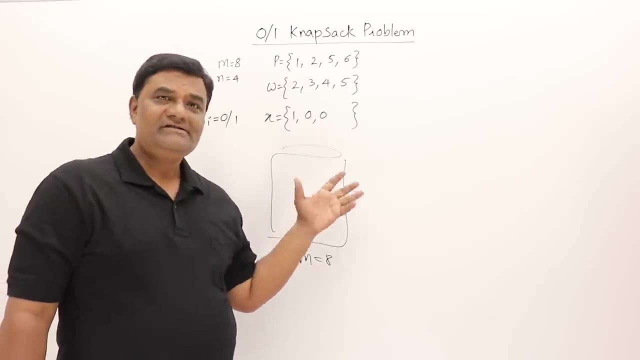 that the object that I am going to carry are not divisible, breakable, So I cannot take the fraction of that object. So this means these are some solid objects, Maybe a mixer or microwave oven or a router, It can be something like that. So I have to write down which one. 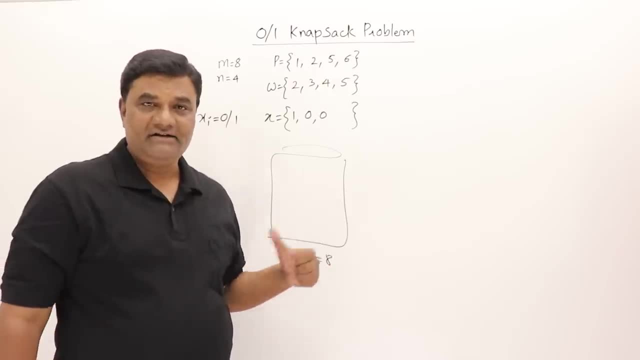 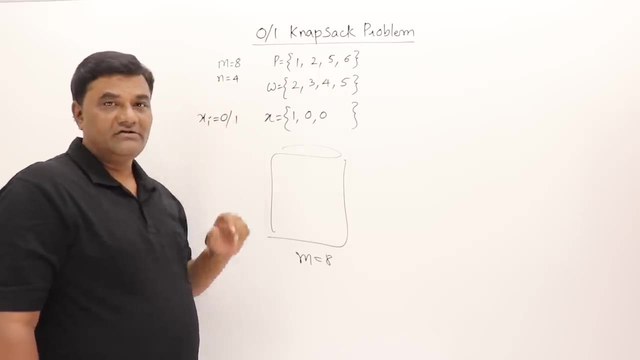 is included and which one is not. So I have to write down the value of the object like this, So I can write down half of the mixture in the bag. So these are indivisible objects. So either I should carry the whole object or don't carry it at all. So I have to carry. 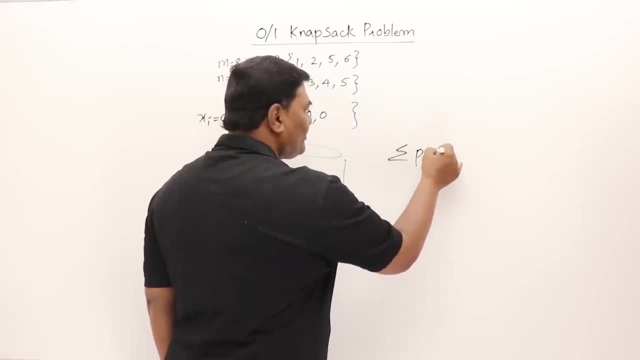 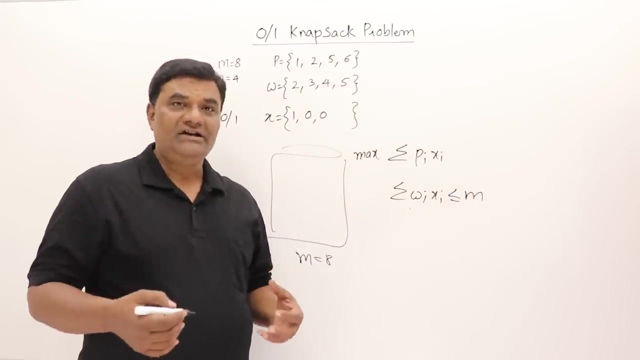 the object such that the sum of their profits should be maximized and sum of their weights should be less than or equal to the capacity of the bag. Now let us know the approach of dynamic programming for solving this one. Now, few important things about dynamic programming. 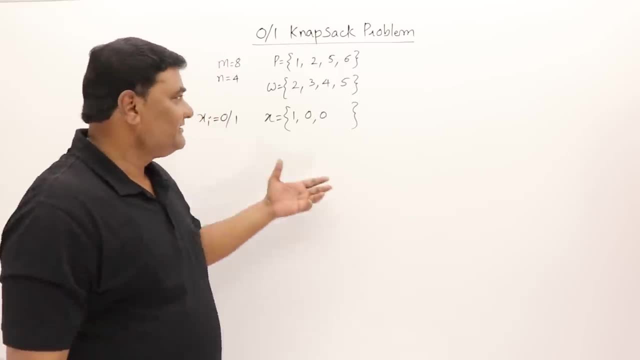 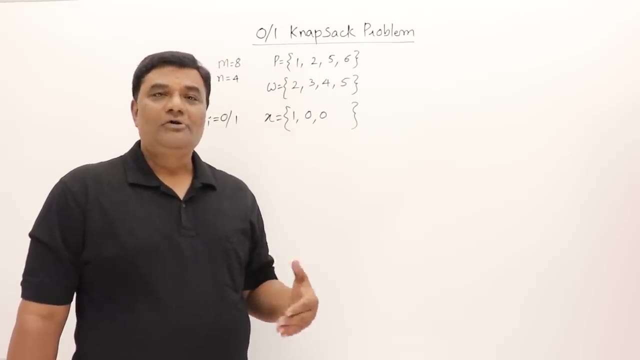 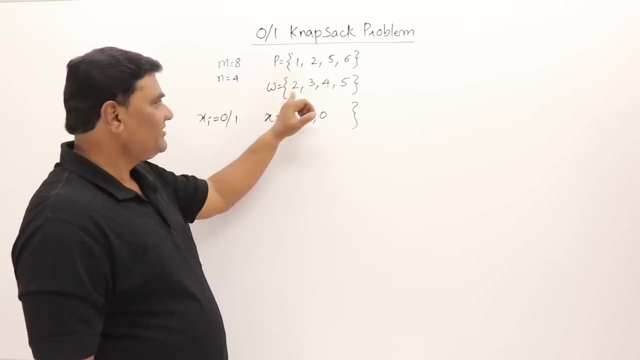 Dynamic programming is useful for solving optimization problem. Yes, this demands maximum results for its optimization problem. Second thing: dynamic programming says that the problem should be solved in sequence of decisions. So yes, we can take the sequence of decisions for every object we can take. shall I include or not, include or not include or not? So 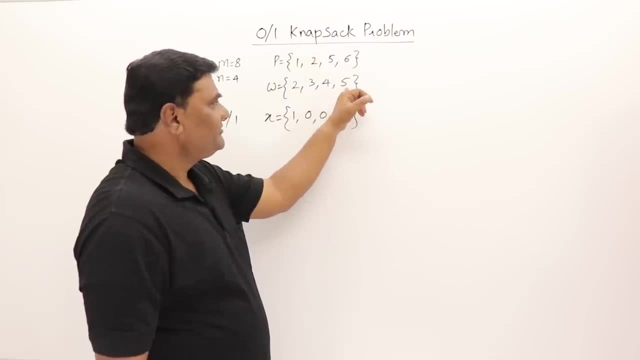 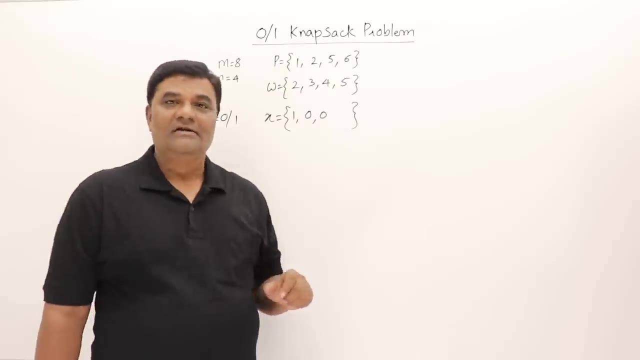 I can take decisions. I can even start taking the decision of the last object also include or not, include or not. So usually in this one we take the decision from last object towards first object. So we can take sequence of decision. Next thing: one more point that 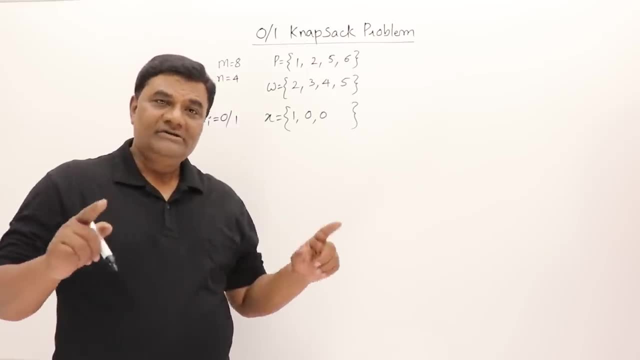 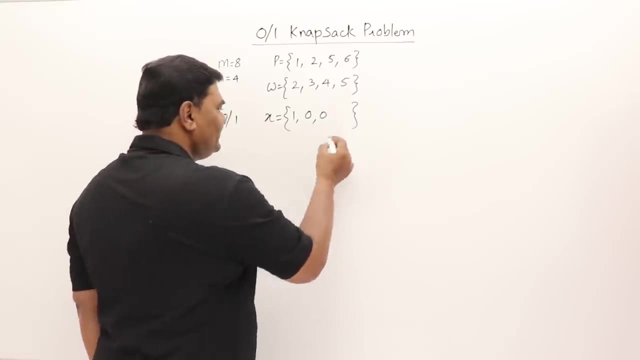 dynamic programming says that you should try all possible solutions and pick up the best one. Now, how many possible solutions are there? See, when I am writing the solution in the form of zeros and ones, then it can be zero, zero. zero means no object is included. So 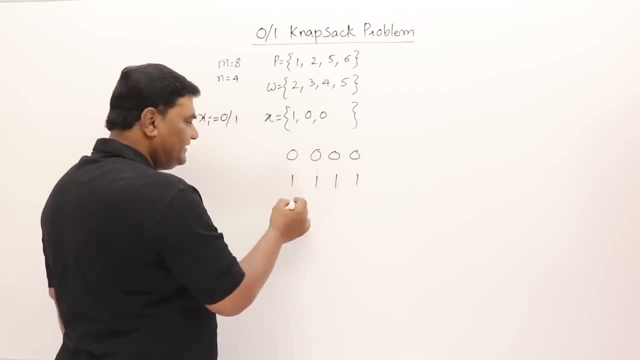 one, one. one one means all objects are included, or zero, zero, zero one means only fourth object is included, or first object is included, or first two objects are included, Like this. there are many possible solutions and some of them may be feasible, some may. 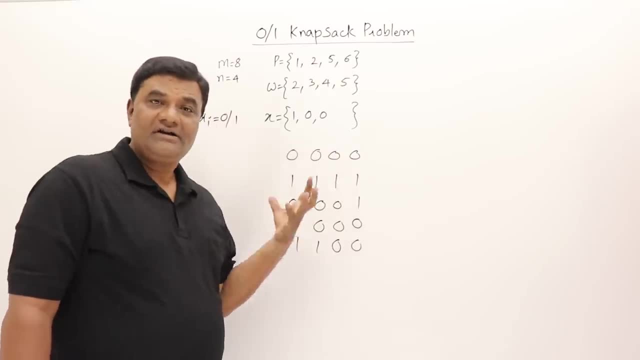 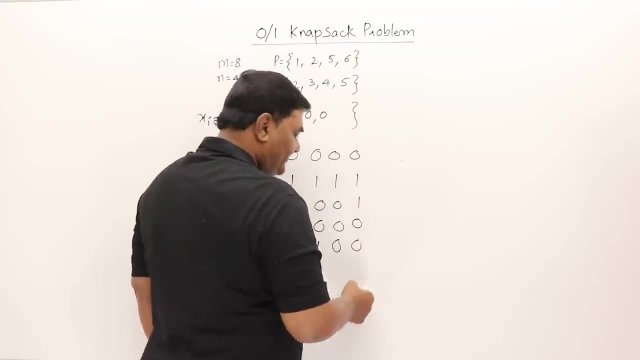 not be feasible. like all objects I cannot include, So anyway I should try all of them and pick up the best one. So, total, how many solutions will be there? So like four zeros and ones form. if I continue So, I will be getting two power: four, five, six, seven. 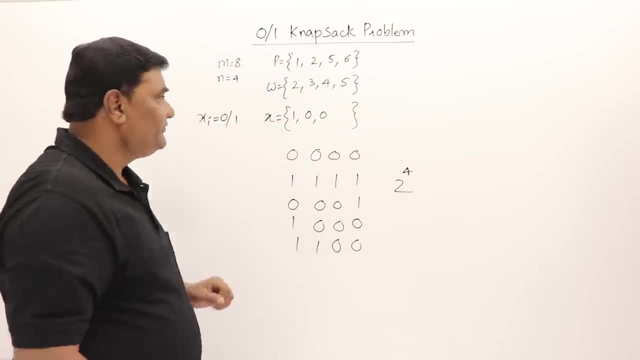 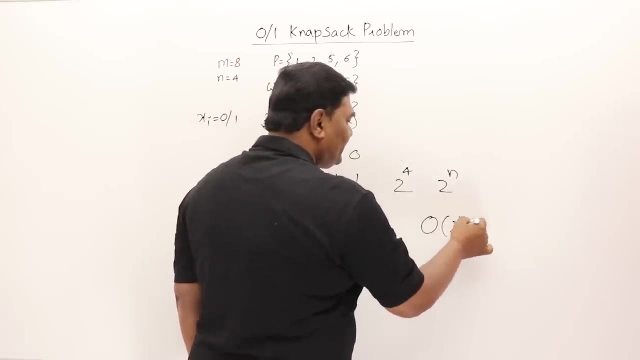 eight and a half, eight and a half. Now again, I should try two power four solutions. So I should try two power four solutions For n objects. it will be two power n solutions. So if I try out all, then the time complexity will be two power n. This is too much time. 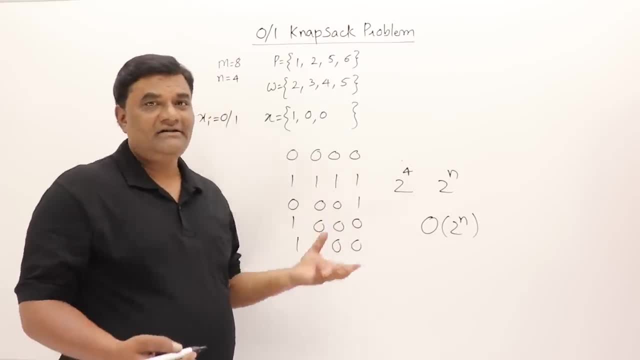 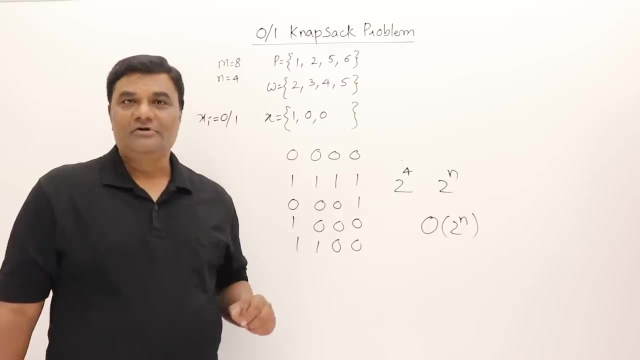 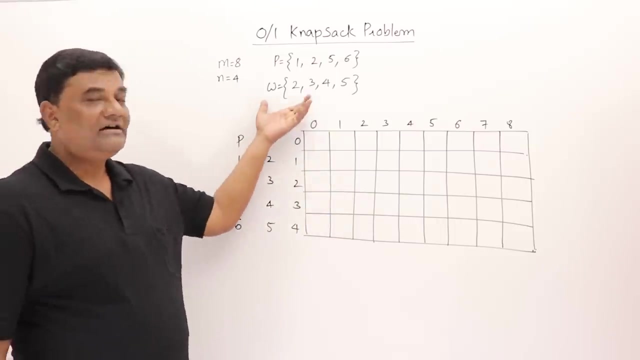 consuming. So dynamic programming shows the easy method for doing the same thing. We will not. we will be indirectly trying all two power n Right, but not directly. So we will not spend that much time. method: let us see how to fill this values and how to get the solution for. 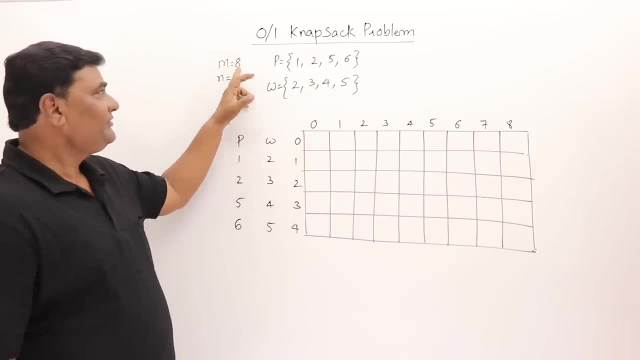 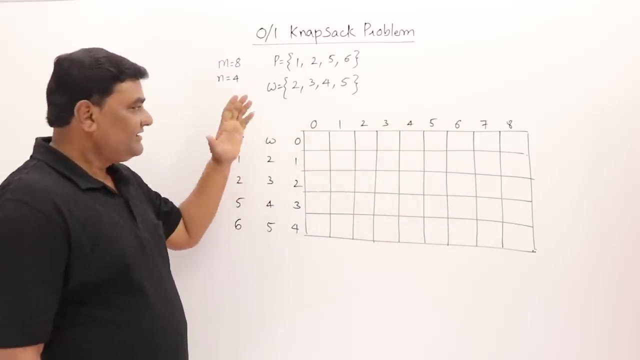 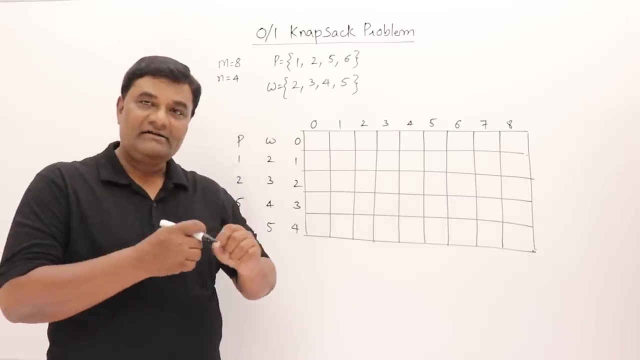 this problem. so for solving, as the capacity of the bag is eight, so I have taken the columns starting from zero to eight. so this means that though the capacity is eight, but will not consider that eight at once, so we'll add weight one by one. so starting from zero, then let us assume weight is one, weight is. 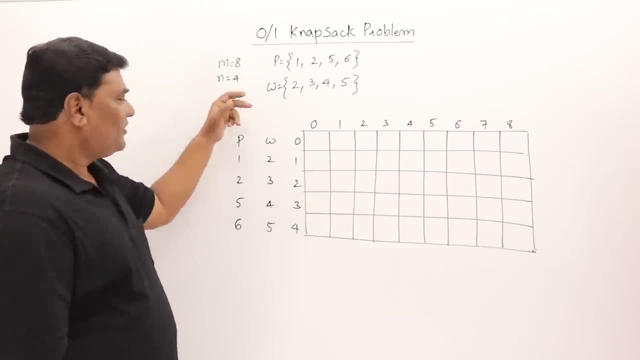 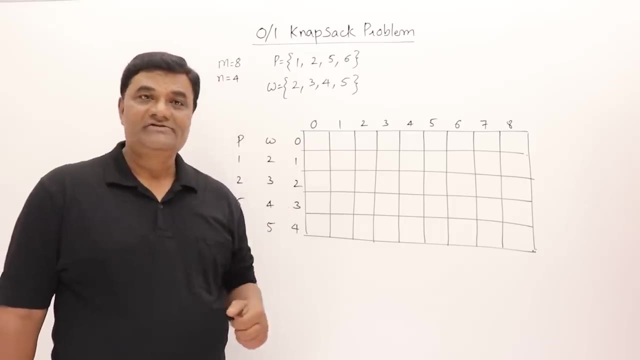 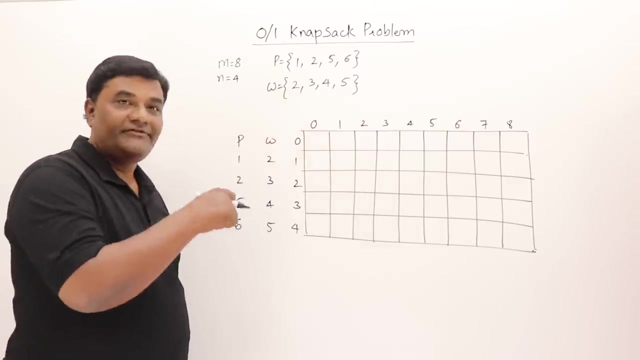 two and so on. then rows, four objects. so I have taken five zero one, two, three, four, so starting from zero. so it means one by one we will consider the object. so initially we will not consider any object, means will not include any object in the bag. so for filling this we have a formula. so I will show you formula after. 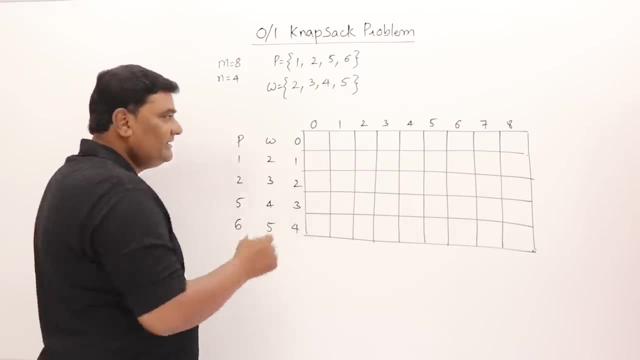 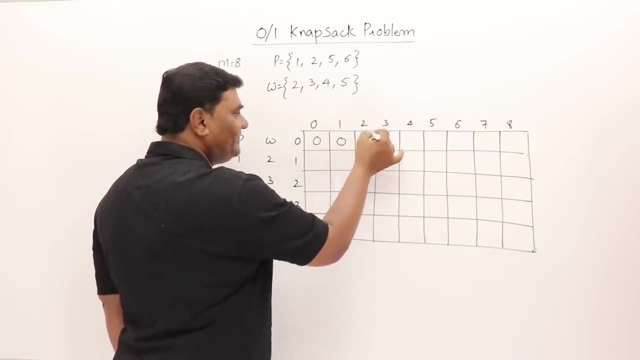 some time after filling some values. so let us see first row as a zero object. no object is included. then what will be the profit? so in these boxes I will be writing the profit. so there is no profit gained when no object is included, and even when the 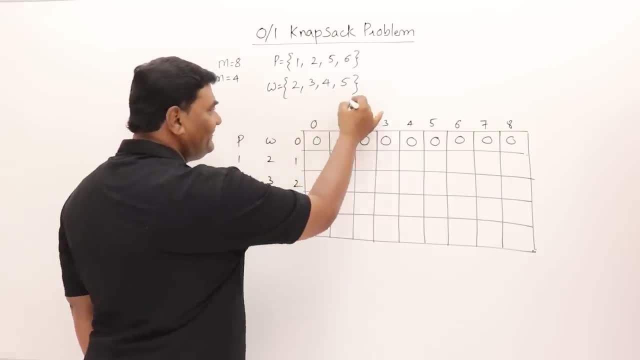 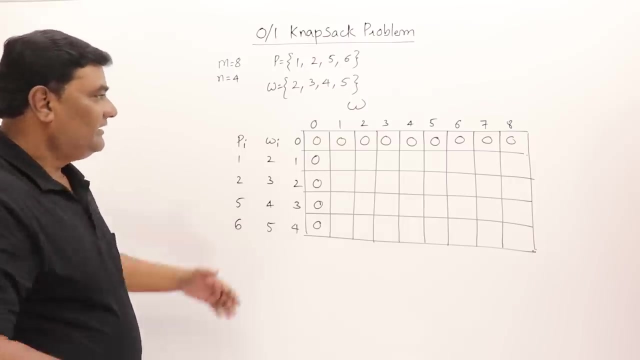 capacity of the bag is zero. these are the, this is the capacity, these are the weights, right, and these are weights and the profits of the objects. so these are the weights and there is then zero weight. is there then? all these are zero, zero, zero. next, now I will start filling, so for that I will consider first object. 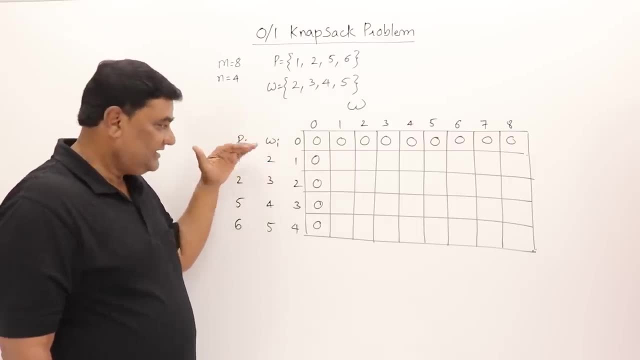 when I consider first object, I'll take this row and I will ignore all other objects, and similarly, when I go to second row, I'll ignore the remaining and I will take the second object as well as the first object and consider the first object also. so it means whenever I am in ith row. 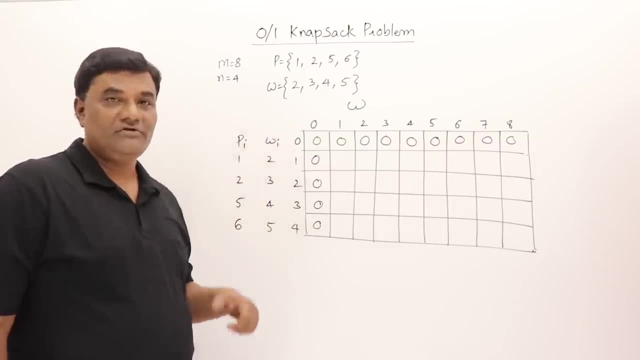 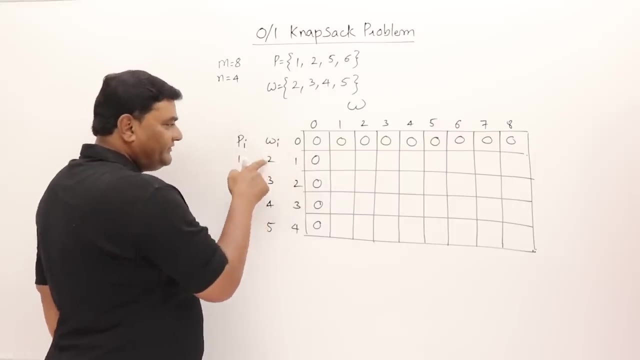 I will consider all the objects in the previous rows also. so for the first row directly, I can fill it. let us see, first row: what is the weight of the first object two? so it can be filled only with the weights of the objects. now let's see. 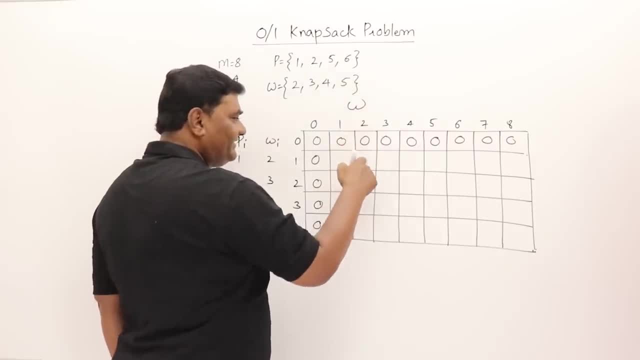 two, so it can be filled only with the weights of the objects. so it can be when the bag capacity is a 2, so here. so what will be the profit? one, so fill one here. then this means this is same value, previous value. usually we write previous value only if required. then 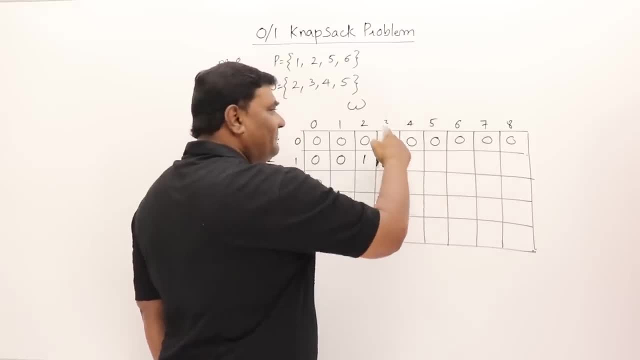 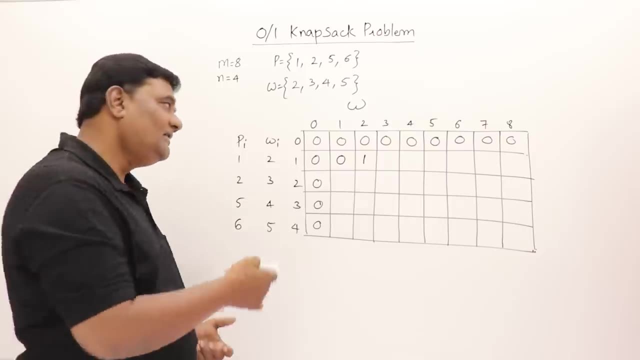 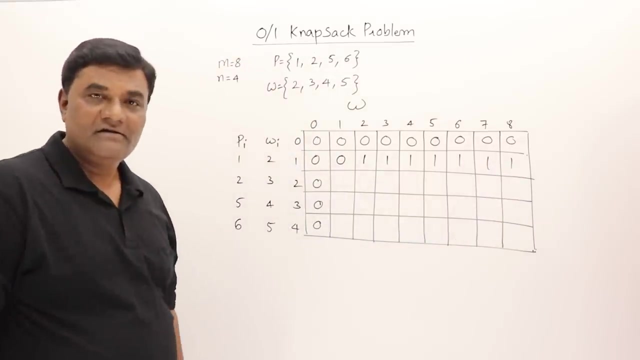 rest of the cells. the capacity of the bag is increasing. but how many objects? i am considering only one, so i don't have anything more to fill in the bag. so only that object i can fill and will be getting profit as 111 only. i'll fill the second row, also right, third row, also in the same. 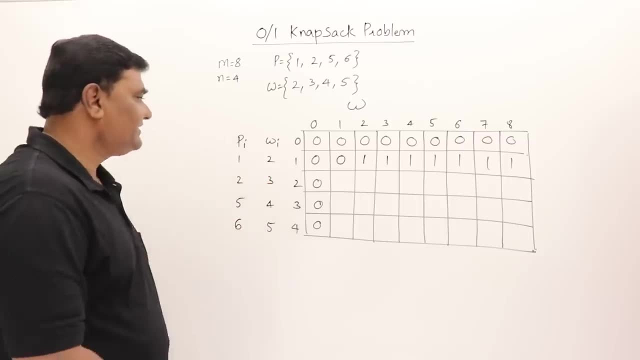 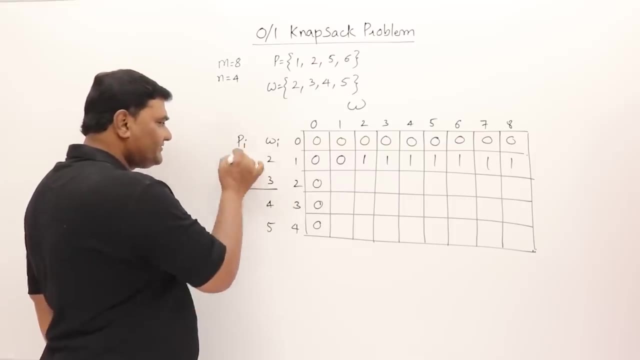 way. then i will write on the formula. let us go to second row. i am going to consider second object. so, as i said, when i consider second object i should also include the first object. so first let us look at the second object. see, the weight of the second object is three. it can be filled. 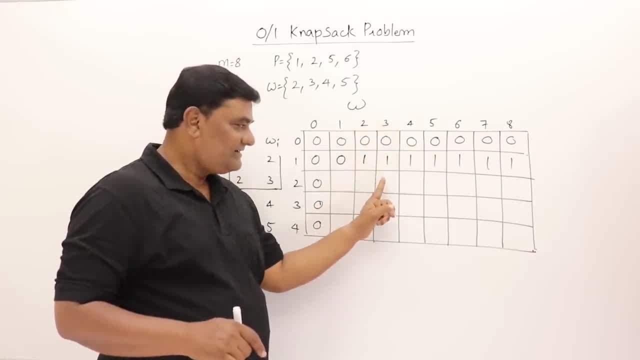 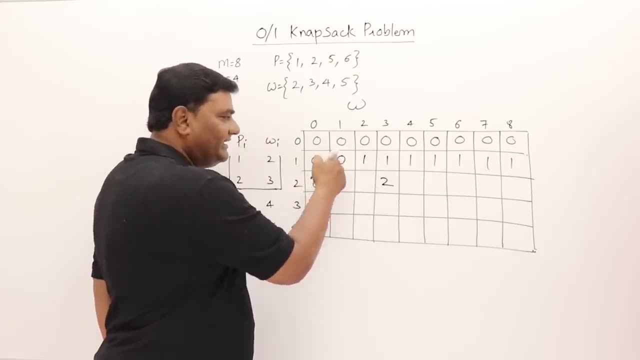 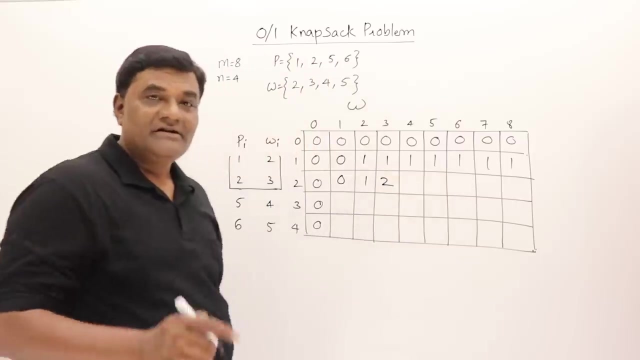 in the bag only if the capacity is a three, so in this cell only it can be filled. so what is the profit? that i'll get two. so put two here. what about this side? it will be same value, same value as the previous row. then, beyond this, what should come here? so as 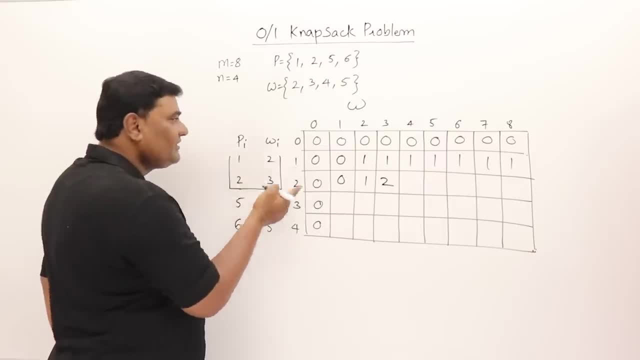 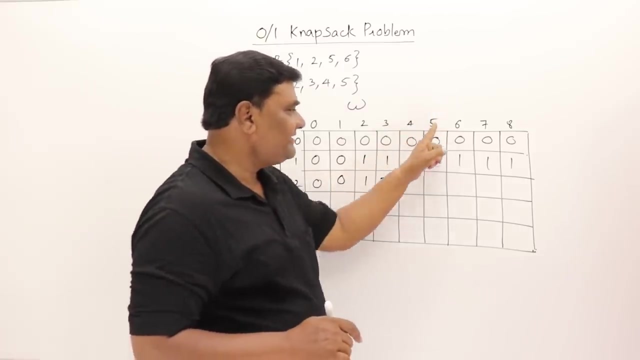 i said that when you are taking second object you should also consider first object. so if i fill the second object also in the bag, total weight required is how much five. so this is five and total profit will be three. so both the objects can be filled when the capacity is five and the total profit will be three. so here both of 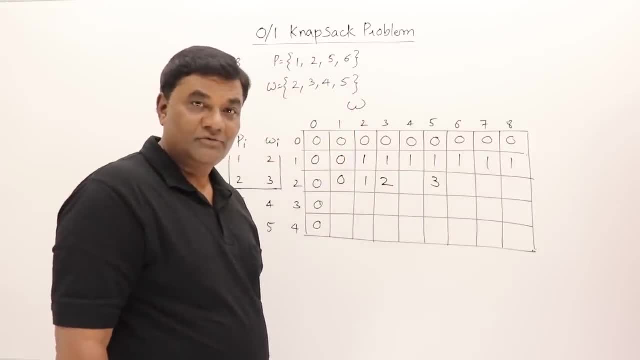 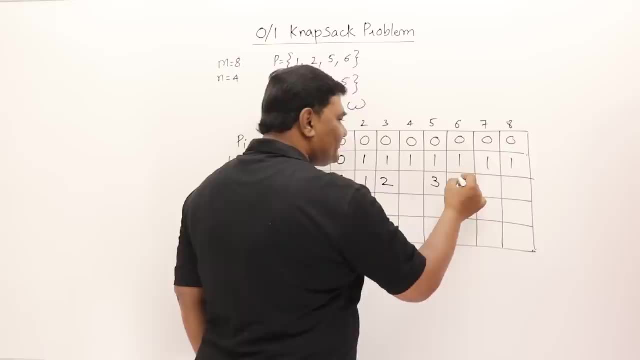 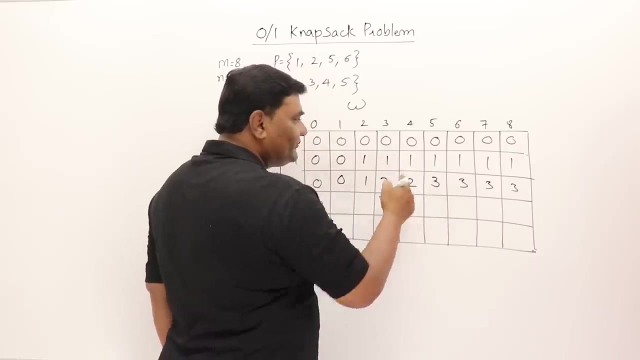 them can be filled. right, both of them. i'm considering both of them. so now i have only two objects and this is giving for both. the objects are filled, so rest of the values will be three, three, three. then what will be the value here? so, as this is two, so this will also be two, so i can. 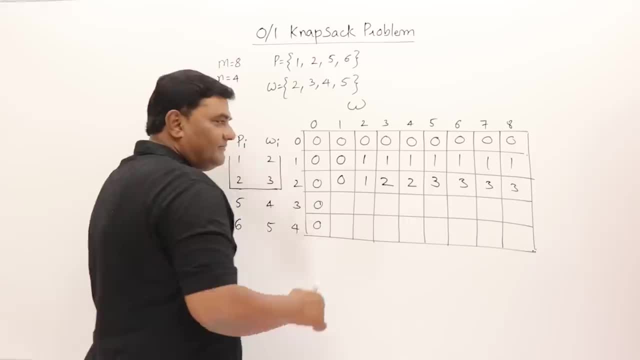 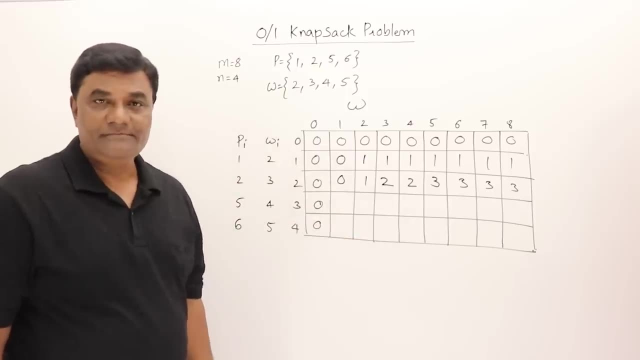 take the previous value or this value, whichever is maximum, i can take the same thing. now i will take the third object also. then for the fourth object, i will show you the formula third object. when i consider third object. if you look at these, the maximum weight is this one and as they are, 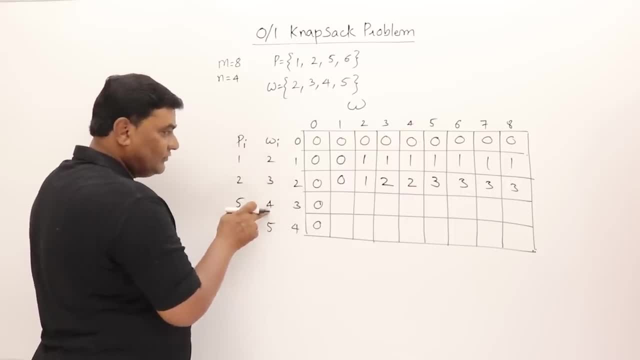 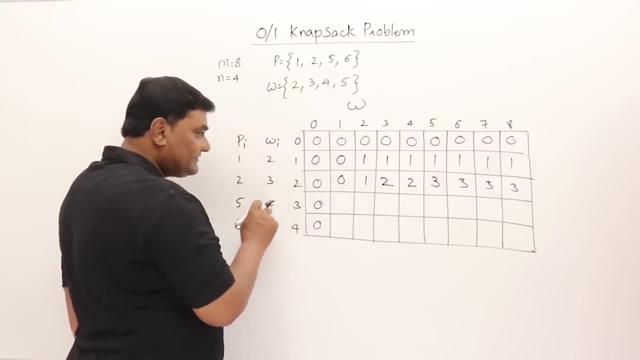 arranged in the increasing order of the weight. so this is: weight is four, so this object can be filled in the bag only if the capacity of the bag is four. so this will be included in the bag when the capacity is four. so the total profit that will be getting is five. so this is five, then before: 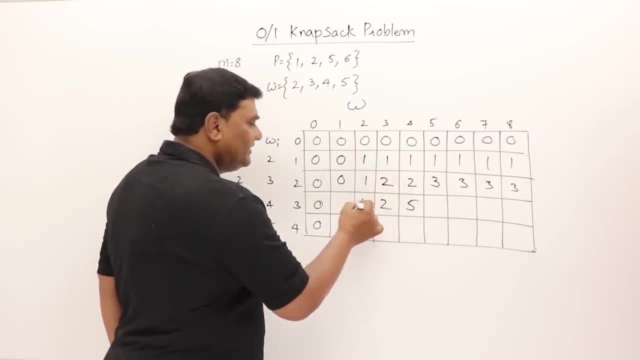 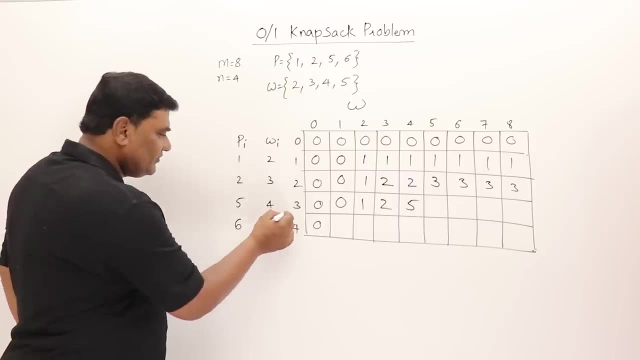 that, whatever the previous row values are. so two, one and zero. now, beyond this, let us see. see. when i am on the third object, i should also consider first and the second object also. so if i just check them, this is four and if i take these two objects it will be total six. weight: weight is six. 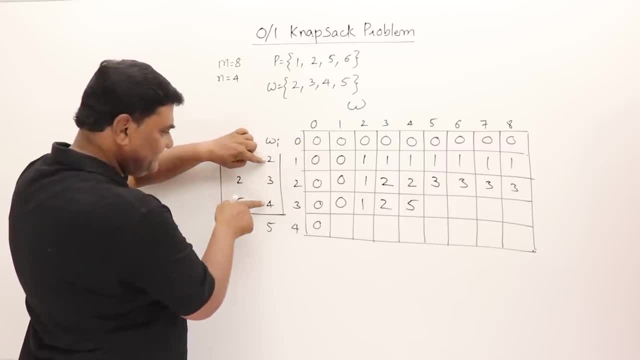 so these two objects i can fill if the weight is six, right. so if i want to fill these two, then these two i can fill when the weight is seven. this two i can fill if the weight is five. and what will be the profit? three, this object itself is five right now. i will consider these. 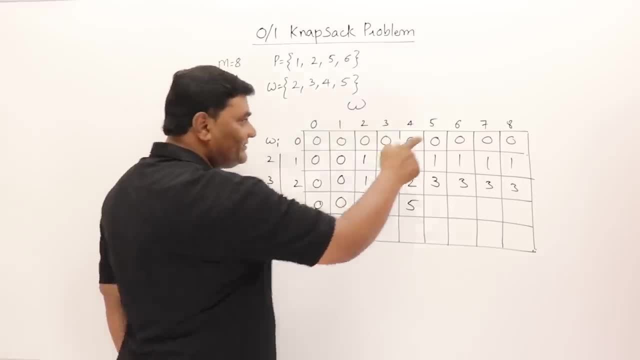 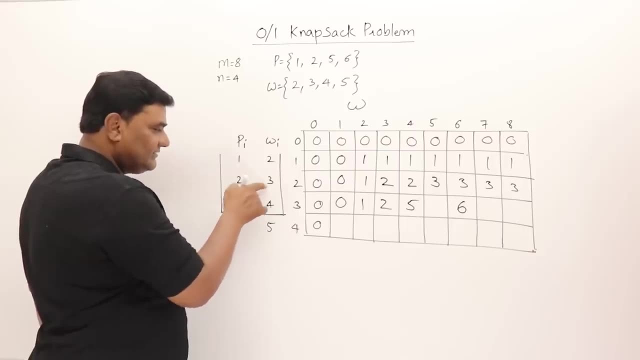 two, six and the total weight will be six. so at six it will be six. only right. and when i consider these two, so total is seven, seven and the profit is also seven. so at seven the profit is seven. can i include all three? it will be ten, but the capacity of the bag is only eight, so i cannot. 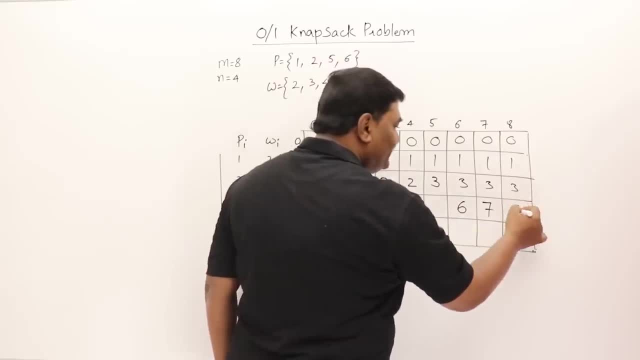 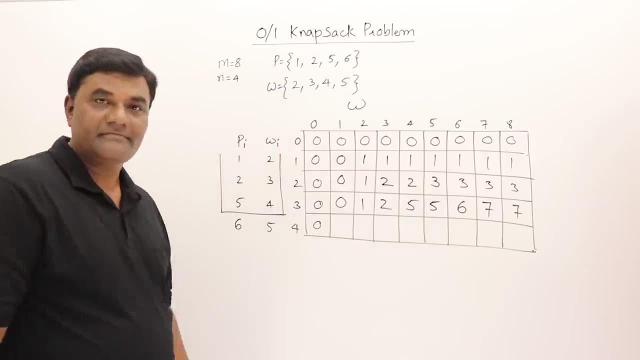 or include all three, then beyond this, the value will be seven only, and before this one, the value will be same as this: five, five, all right. now i will show you the formula and i will fill fourth row with that formula. the formula is like this: if i call this table as v, this table as v. 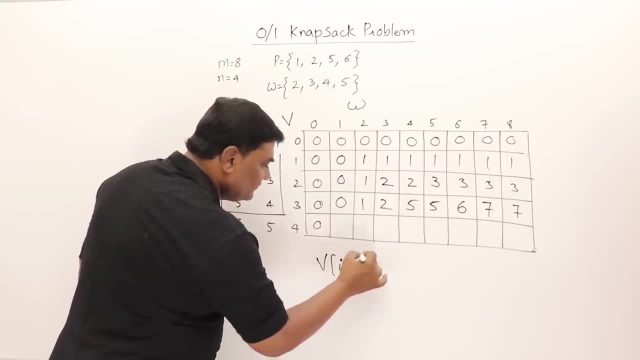 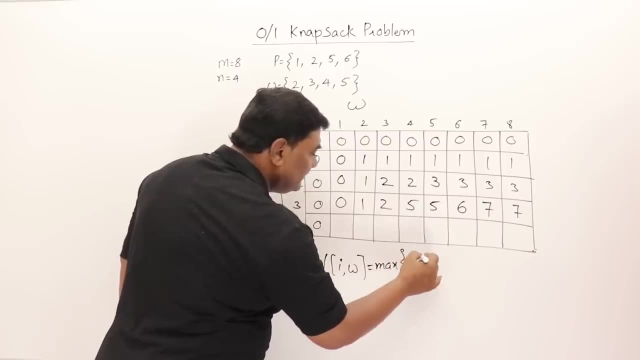 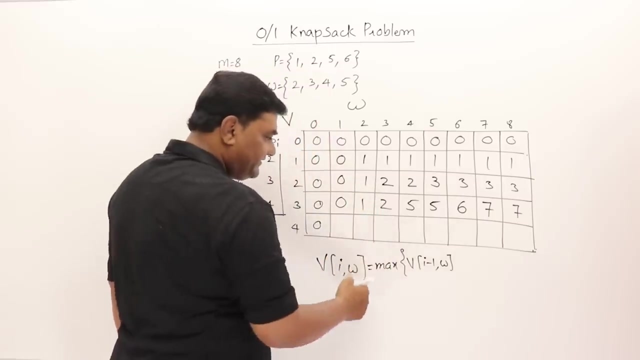 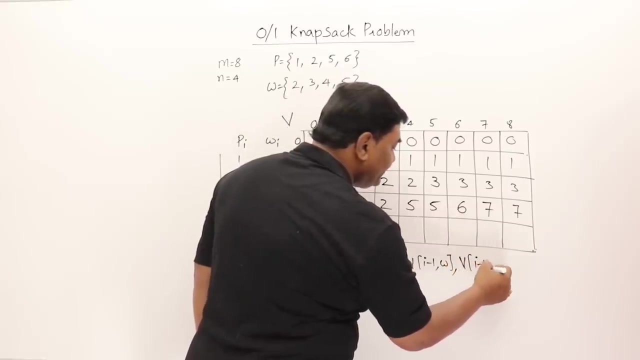 then v of i comma w. i is the row number, w is the column number is maximum of v of i minus one. that is from the previous row i should take. same value means previous row value i should take. this is the meaning or maximum of this one or what v of i minus one comma. weight minus weight of an object. 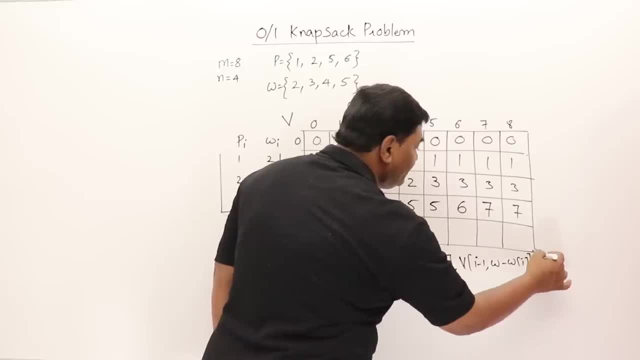 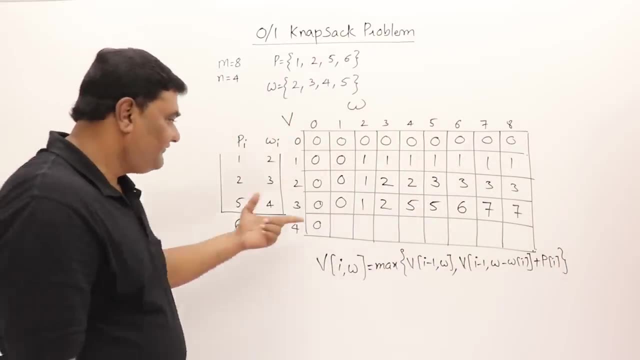 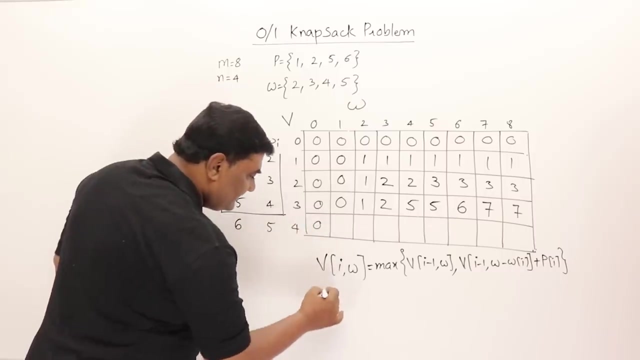 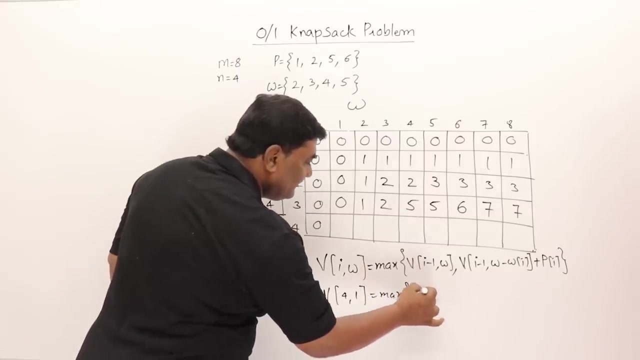 w i plus profit of an object that you are considering. now let us the follow the formula and fill all these. first one, four comma one. i will fill four comma one. so v of four comma one is maximum of v of three comma one. like this is four, so this will: 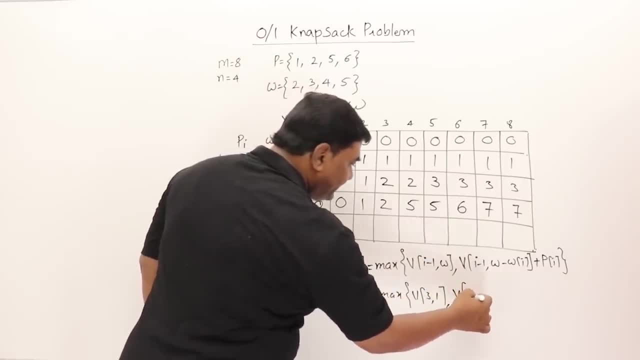 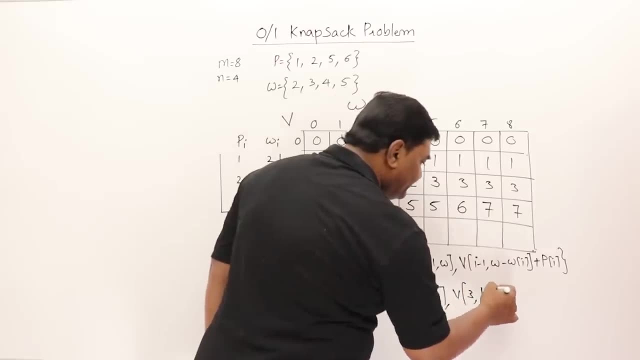 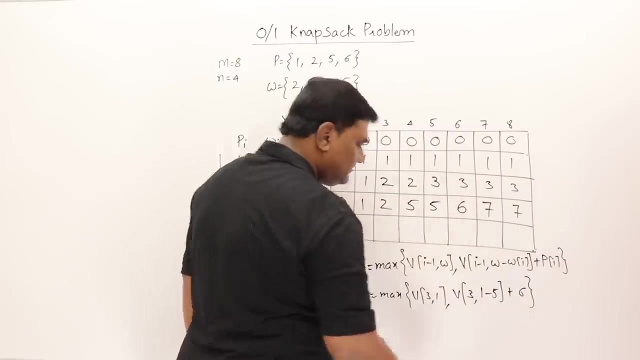 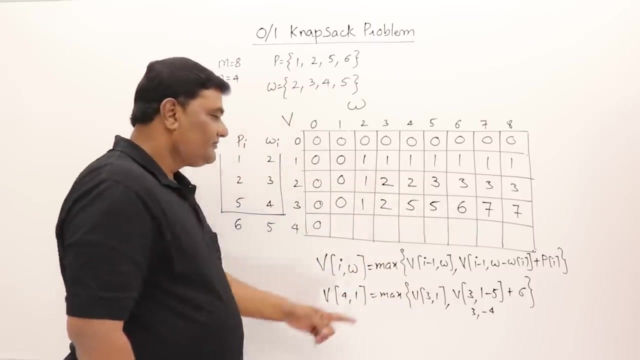 be three comma. v of three comma. weight is how much one minus weight of an object. weight of an object is five, one minus five plus profit of that object is six, six. now this becomes three comma minus four. there is no such location, so that value becomes undefined. so only this value will be defined. v of three comma, one will be: 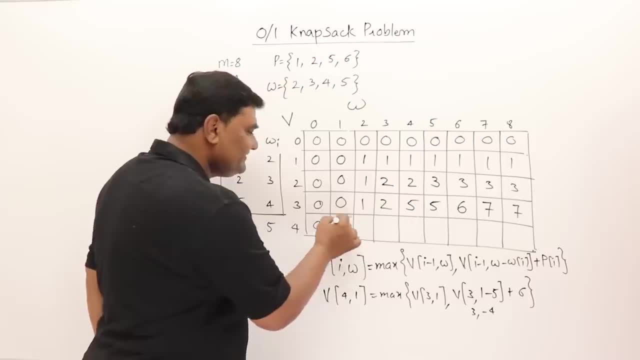 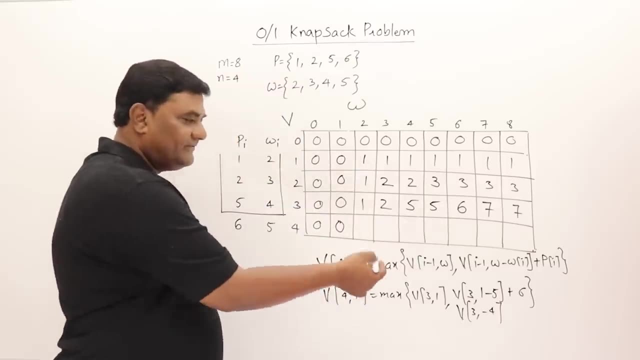 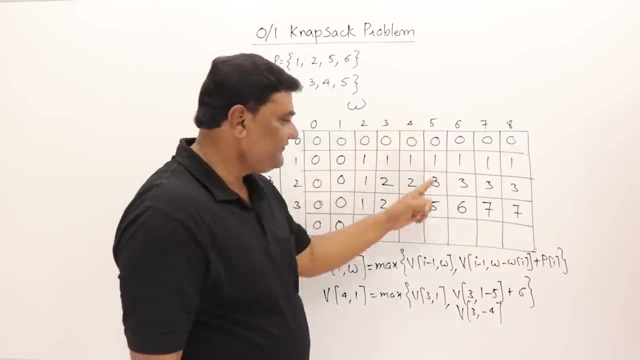 defined. so v of three comma one is what zero? so i should take zero only. there is will not be any such index. v of three comma minus four, yes, for that i have to take zero only. so it means up to what i'll be getting negative numbers up to fifth weight up to fifth. 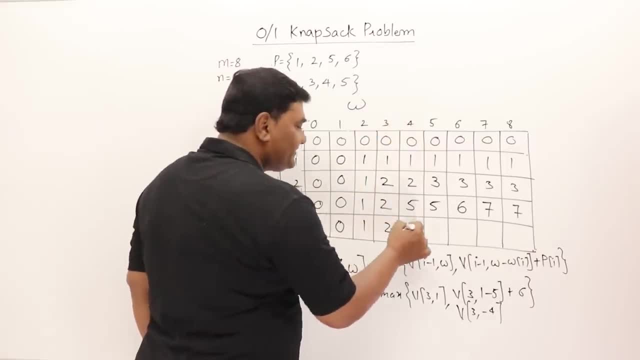 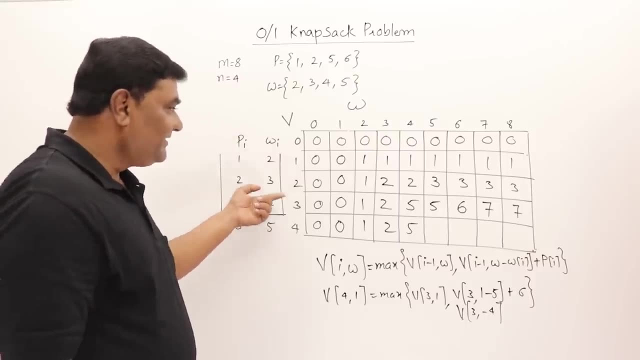 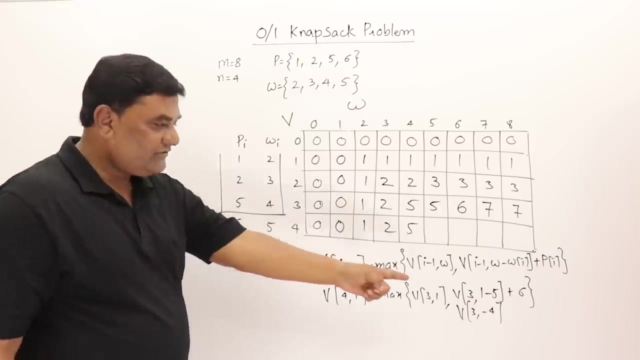 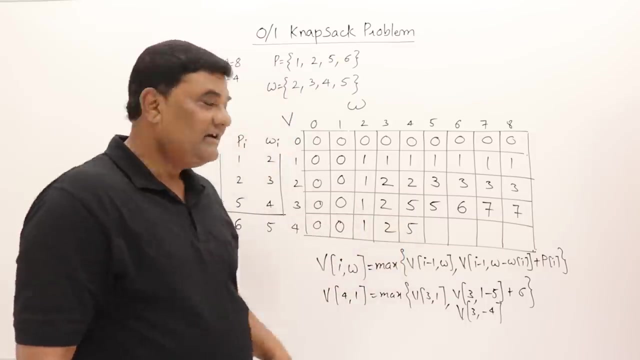 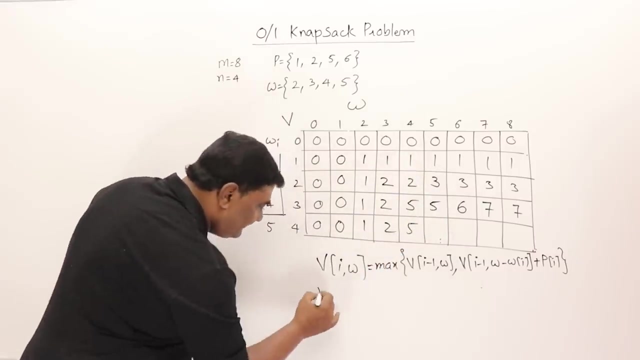 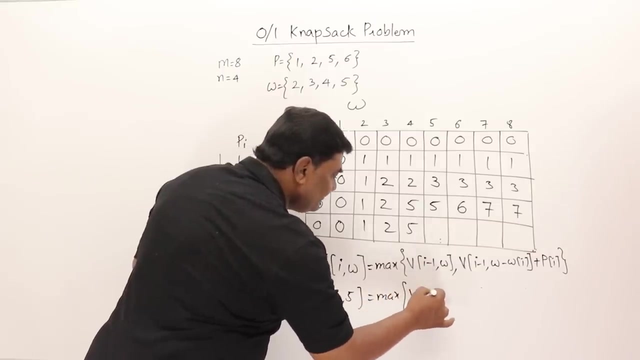 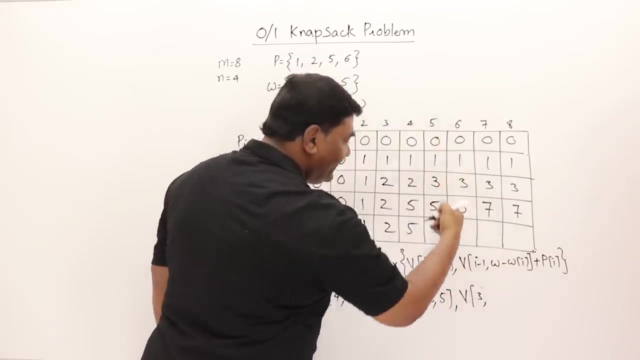 weight. so till here i should fill these values as it is, only so that's what i was saying- that this can be considered, or this can be considered in fourth. so right on its value and all previous values as it is. so the same thing here, because there will be getting negative. so till fifth weight, till fifth weight before that, till before that i have filled, as it is now this fifth weight, how to fill. i will show you, for this value, four comma five, v of four comma five is maximum of v of three comma five comma. v of three comma weight is how much five. 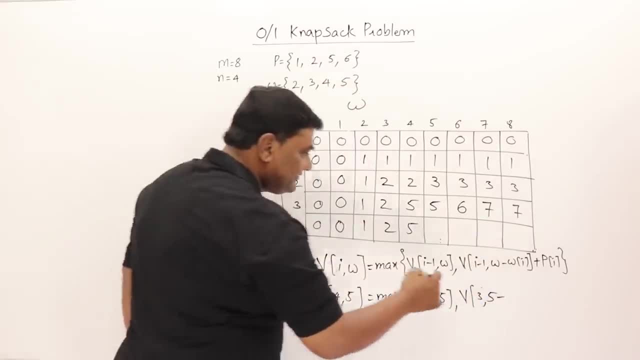 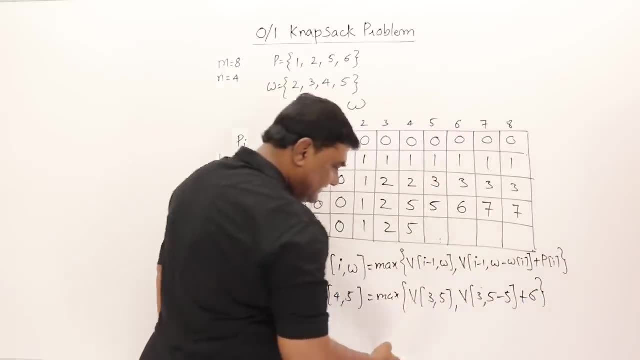 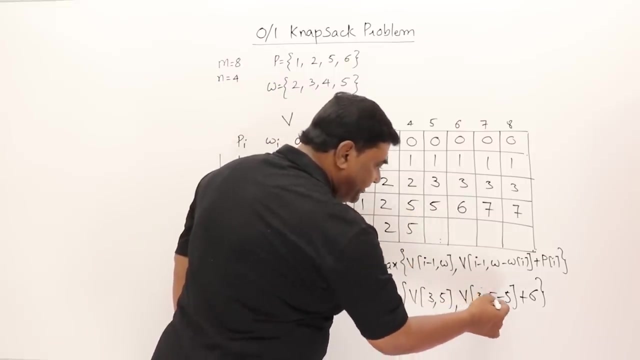 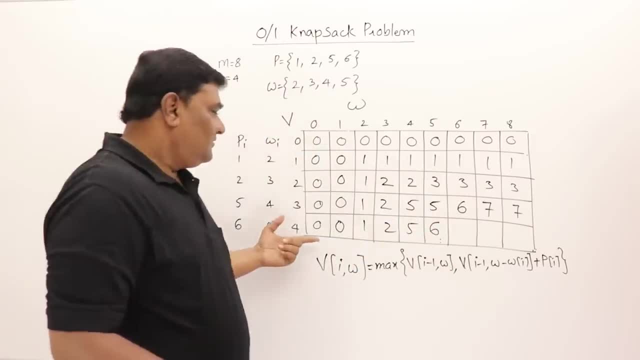 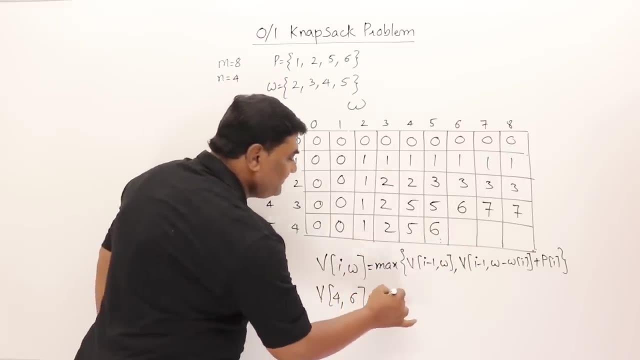 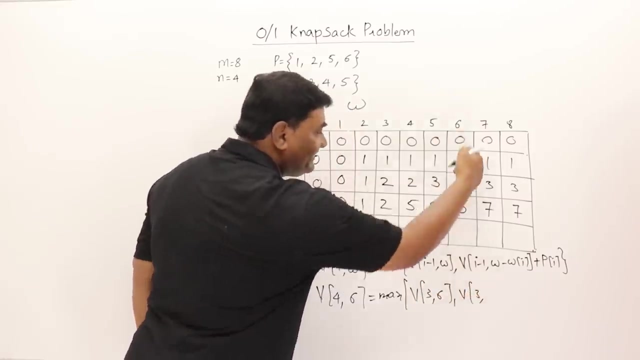 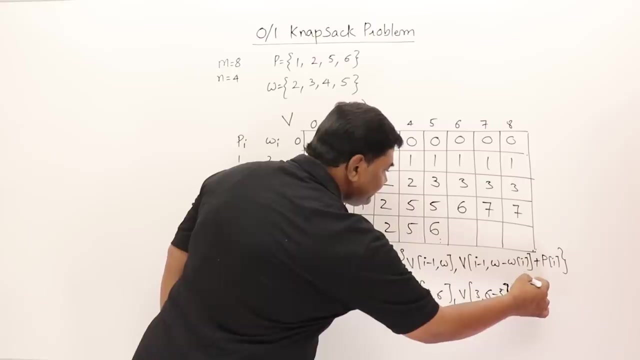 means this object is included here. now, four comma six. i will find out: v of four comma six is maximum of v of three comma six comma. v of three comma weight is six right and the weight of the object is five plus profit of the object is six. so how much this. 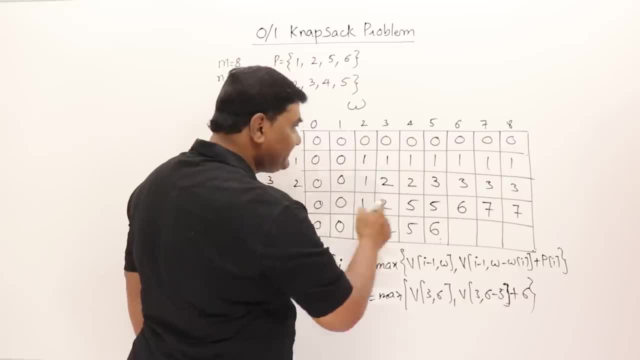 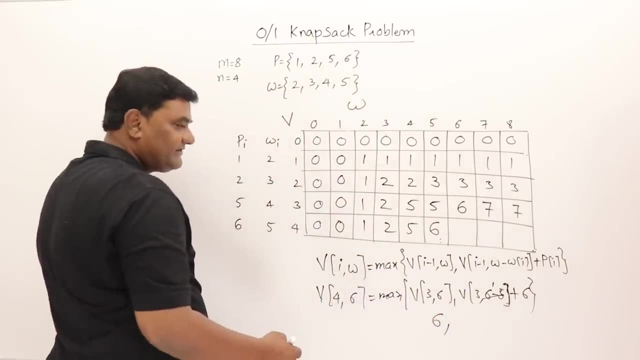 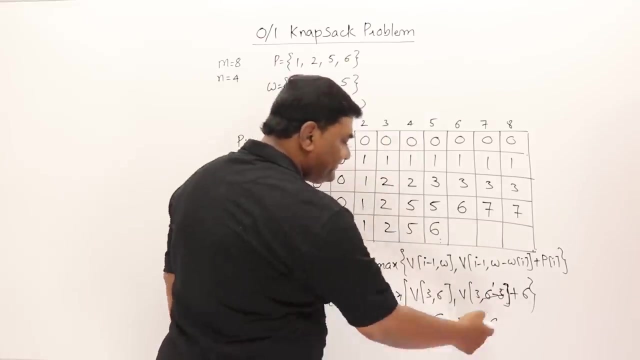 is v of three comma six is how much three comma six, is six six comma v of three comma six minus one, six minus five. that is one three comma one. three comma one is how much zero, zero plus six. so the answer is both are same only. so take six only. 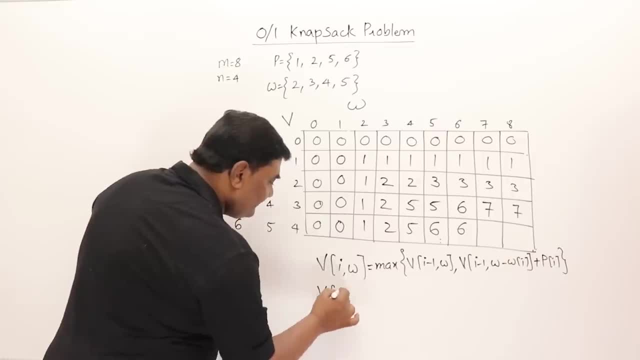 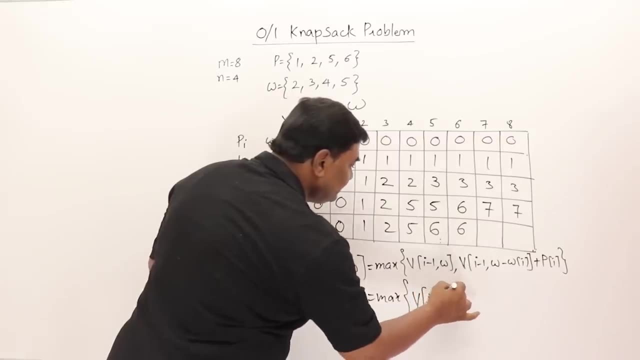 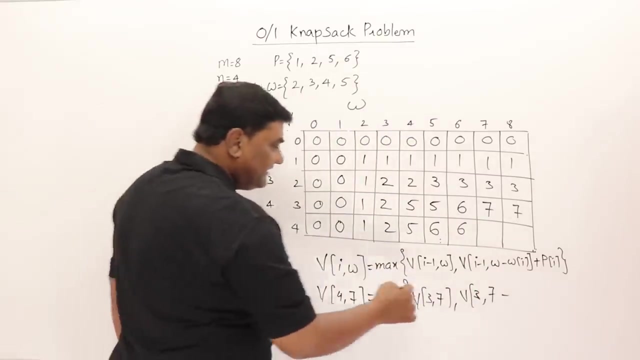 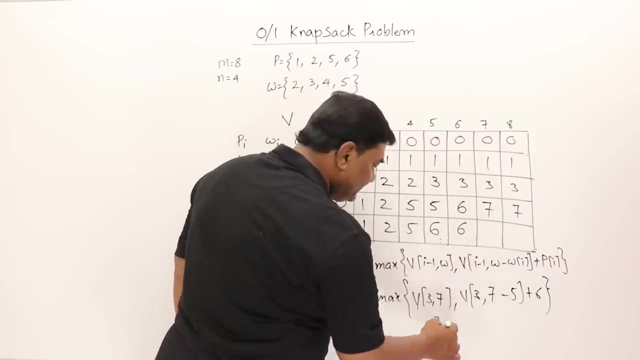 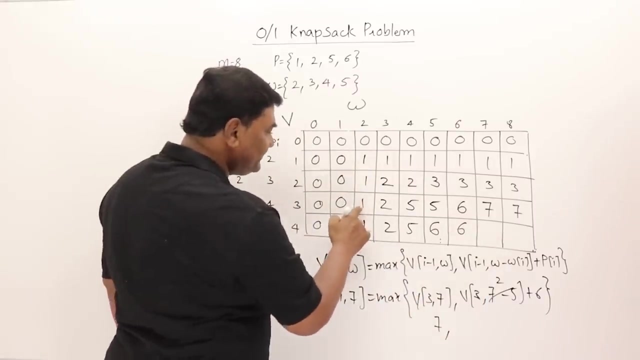 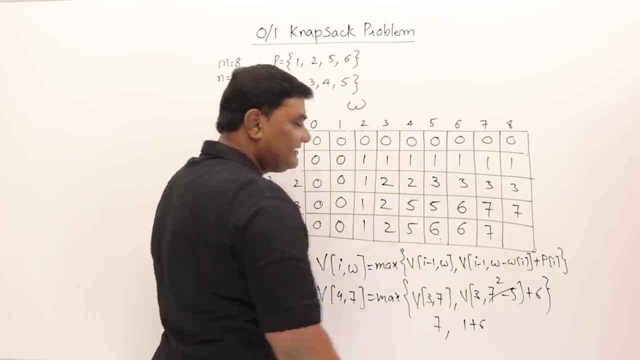 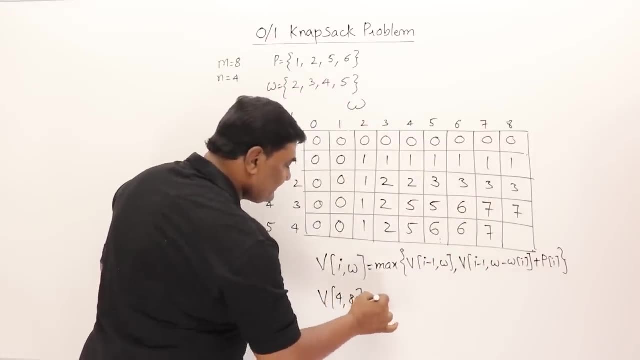 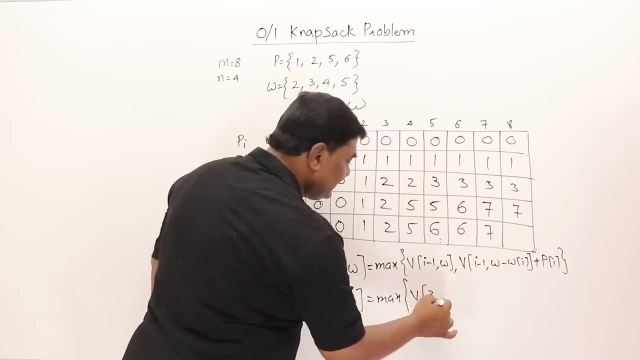 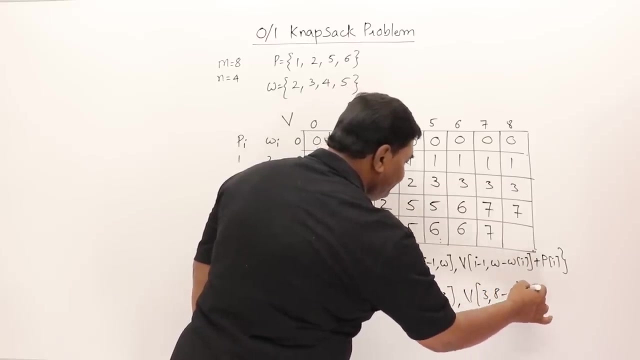 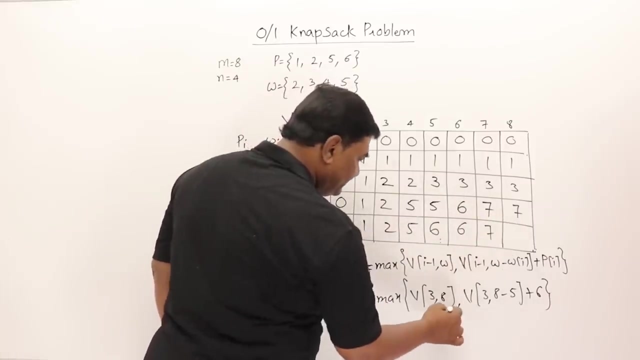 both i am getting seven or seven, so they are same only take seven. v of four comma eight. four comma eight is maximum of v of three comma eight comma v of three comma weight is eight minus. the weight of an object is five plus. profit is six, three comma eight. how much three comma eight is seven. 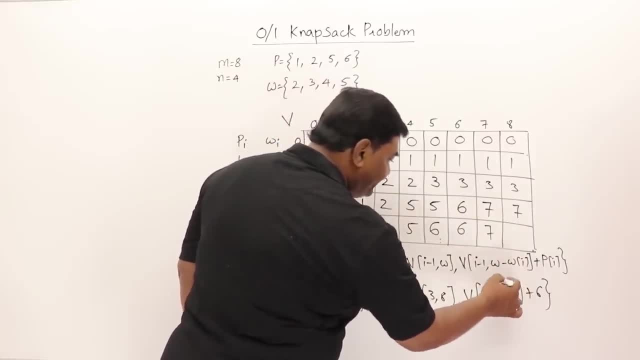 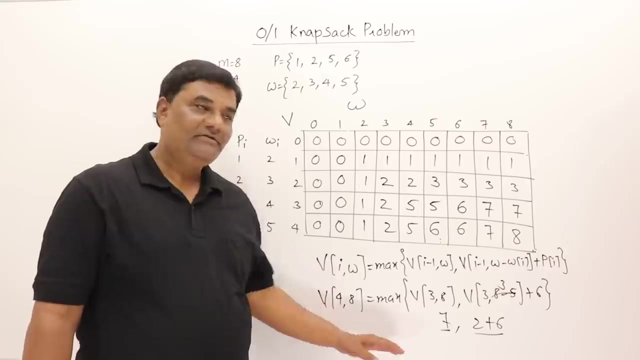 comma v of three comma eight minus five is three. three comma three. how much two? so this is two plus six. so how much this is? this is seven and this is eight. so answer is eight. so this is how the table is filled. so i have used the formula for few cells in the last row. 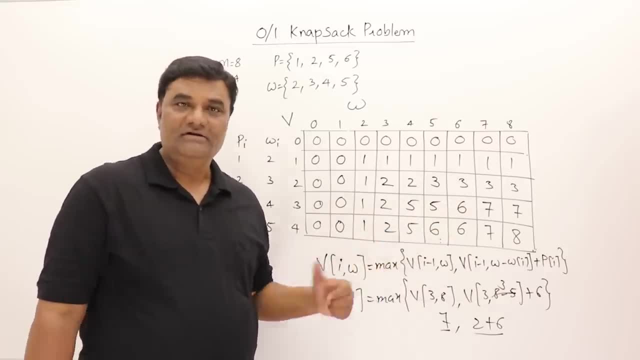 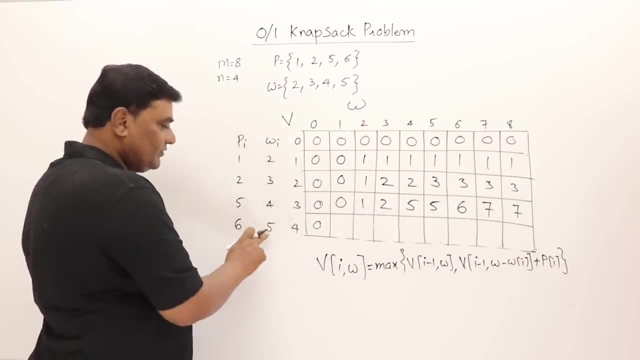 and this can also be filled directly, also without the formula. let me show you how to fill this last row directly. i am considering fourth object whose weight is five and the profit is six. so in fifth column just write six, it's profit. and what to write on the cells before that? same value as the. 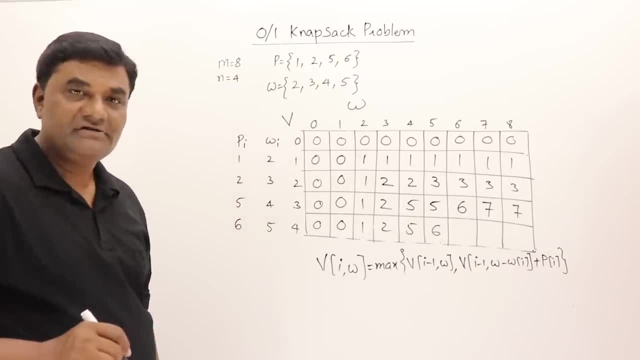 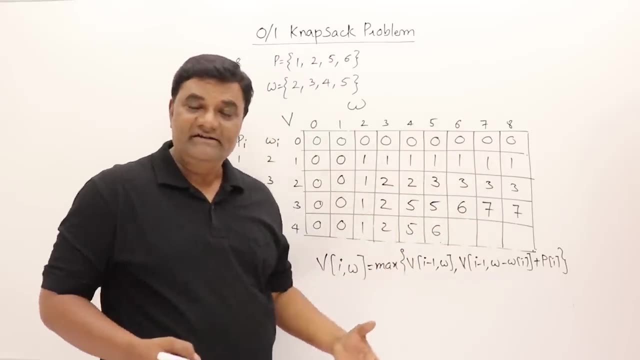 previous row. this what you do first, then beyond this. now the weight is five. beyond this, the capacity of the bag is increasing, so the weight of the bag is increasing. so the weight of the bag is increasing. so i can include other objects also. so let us check other objects, what i can include in the 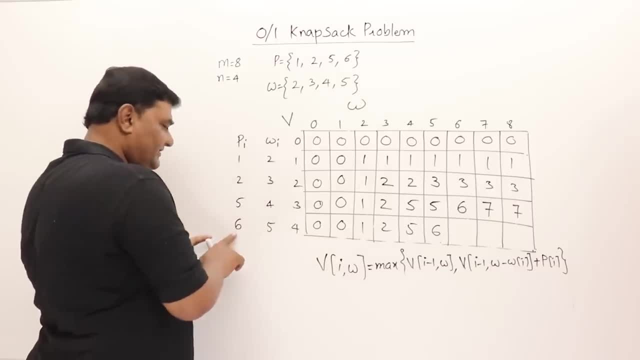 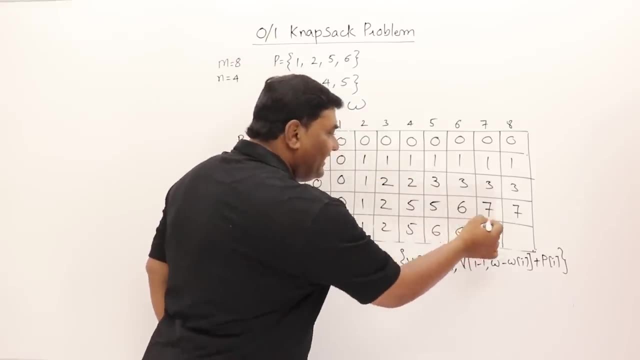 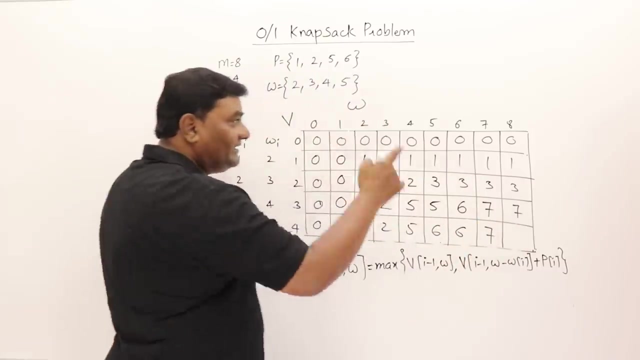 sixth column. this object is definitely because its profit is maximum right. five plus two, seven at six, nothing will happen. so take six. only at seven i can consider these two, these two. so this is six plus one, seven, seven. then at eight, when the bag capacity eight, which of the objects i can consider five plus three? 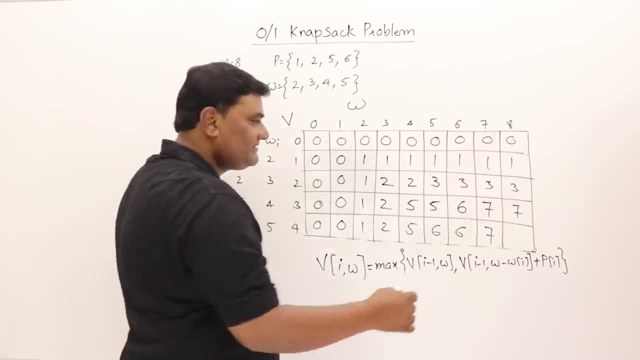 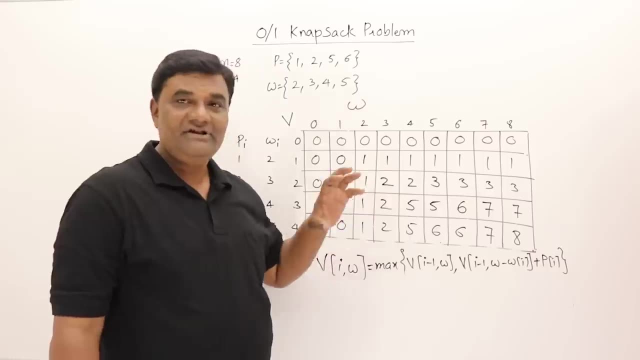 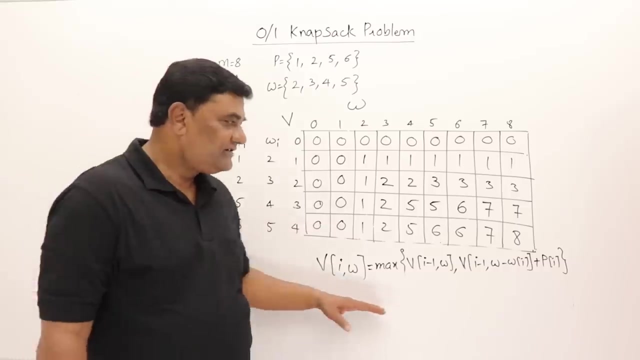 eight, so six and two eight, so this is eight. so whichever objects that you can consider, you just add them and in that capacity, if they are fitting in, you write on the max total profit. so this is a simple method for filling the cells, instead of following this complex formula. 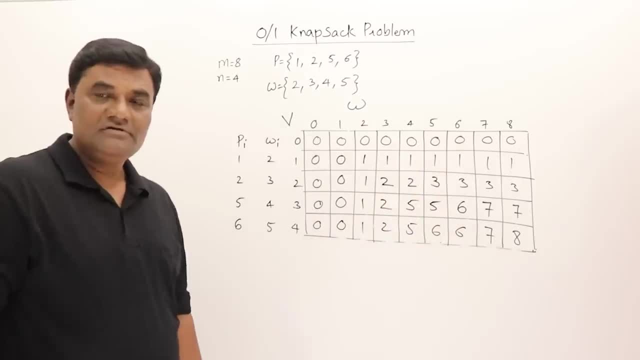 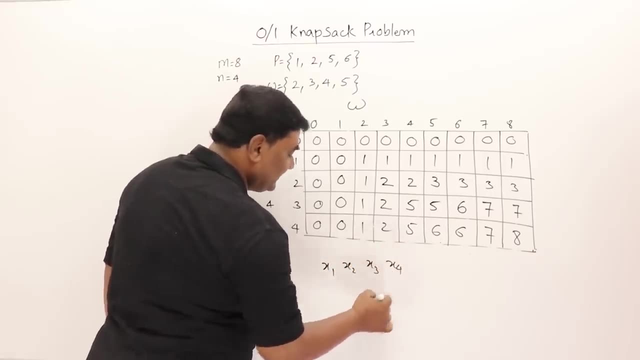 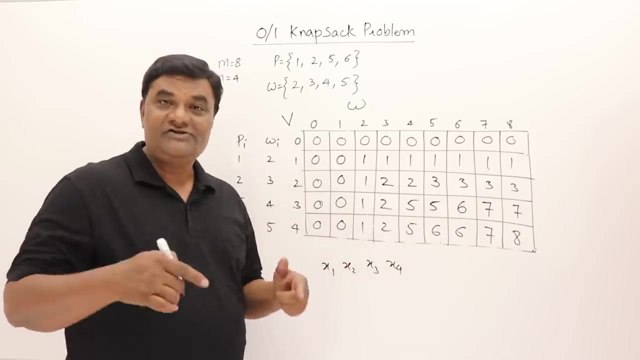 you can follow that method. so i have shown you both solution. i have to write down x, 1, x, 2, x, 3, x 4 values. now these now for finding these answers. actually, i'll be taking sequence of decision. now. see, the decisions can be taken only if you have the data. yes, we have kept the 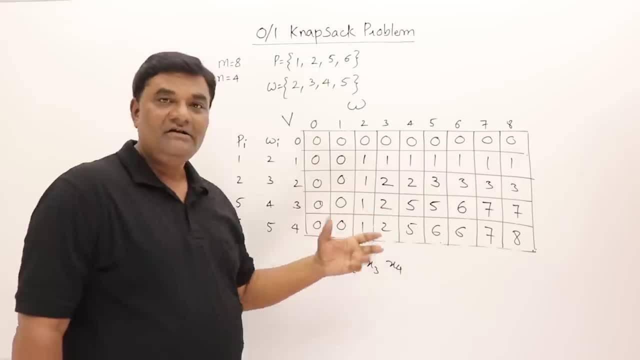 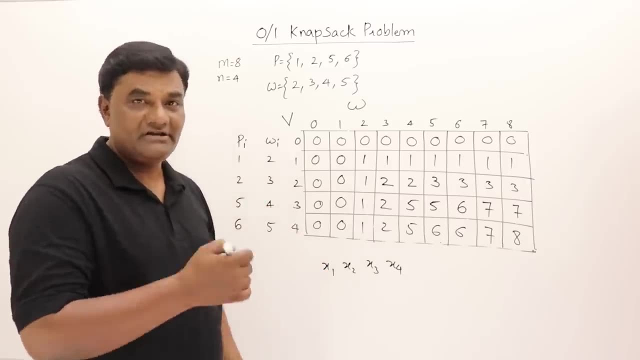 data ready. the formula was used for filling this data. now i have to take the sequence of decisions. so how to solve? so, actually, i have to know which object should be included and which should not be included in the bag. so let us come with the maximum profit. 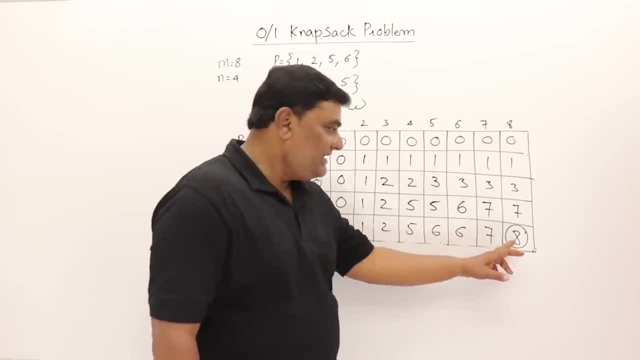 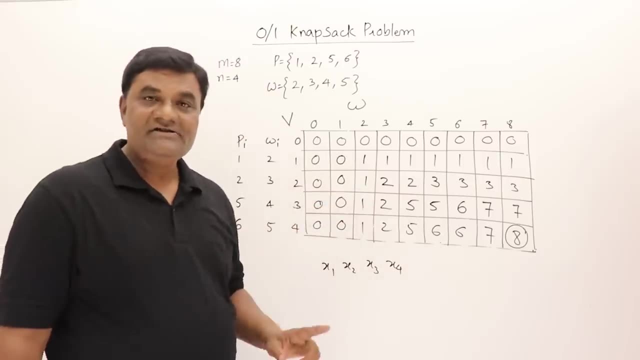 that is eight, the last cell. this eight is generated only in fourth row and in that previous row you don't find eight anywhere. so it means we got this eight because of including fourth object only. so include the fourth object. right profit is eight. fourth object is included because eight is not there in. 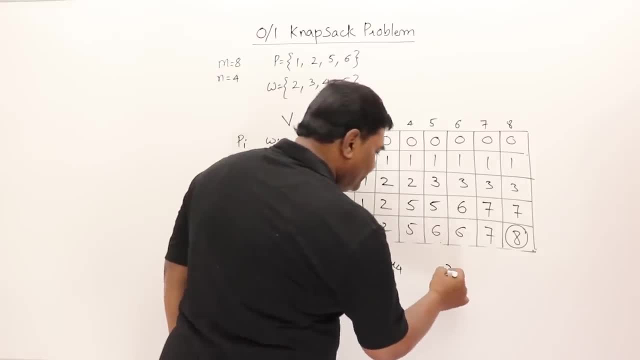 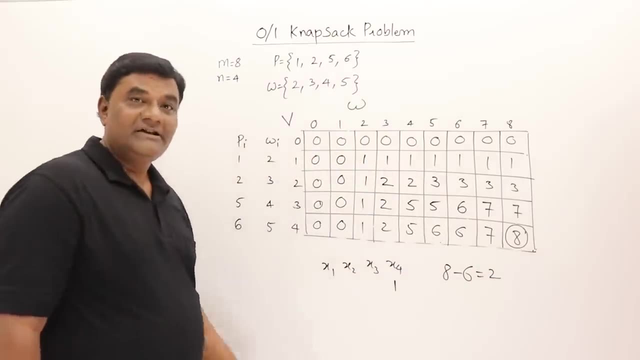 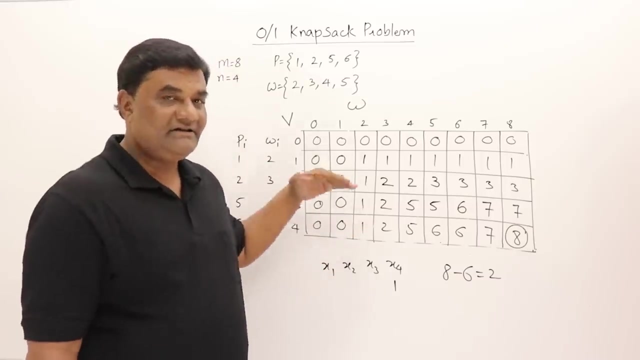 previous row. now what is the profit of the? a fourth object eight minus profit is six, six. so this is two. now remaining profit is two. now check whether two is there in the third row. now i have to check for the third object, fourth, then third, then second and then one. 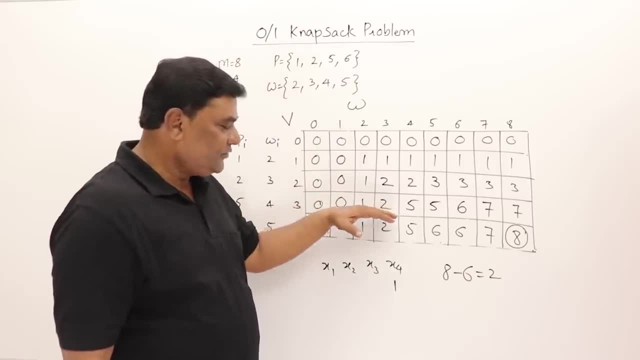 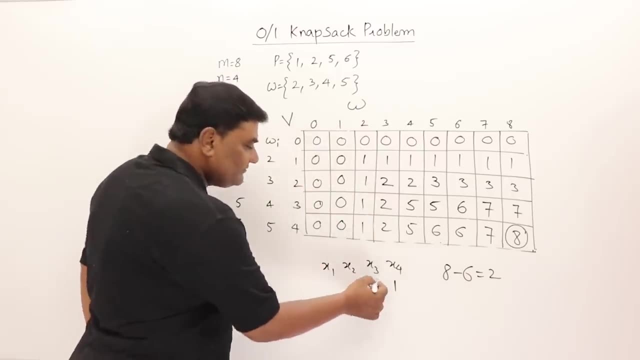 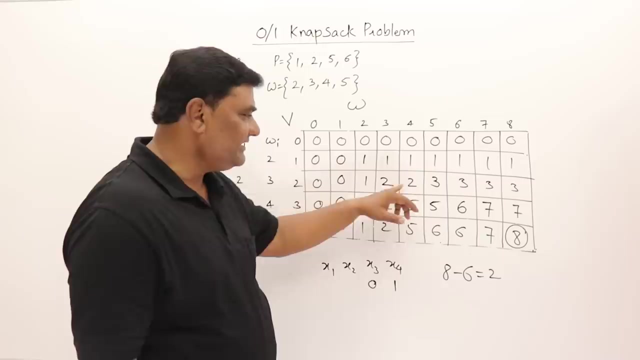 so third object: two is there. yes, as the same value. two is there in the previous row also. yes, it is there. so it means it is not because of third object. so don't include third object. now let us consider second object. is it two there here in the second row? yes, two is there here. 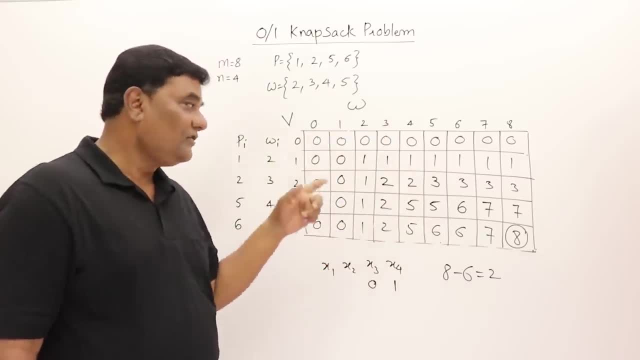 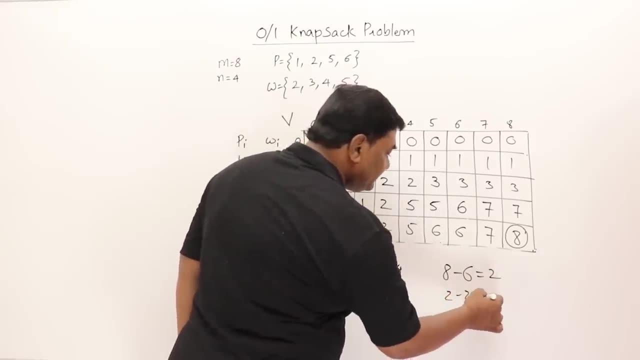 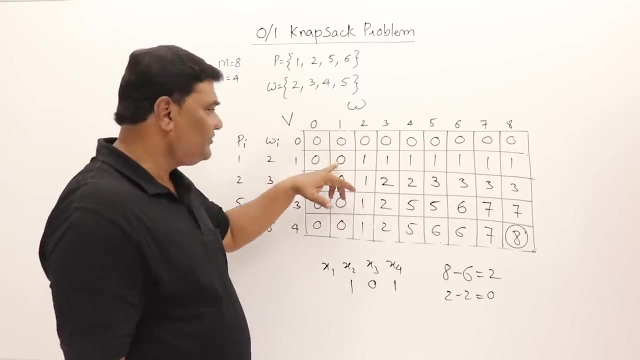 is it there in the first row also? no, so it means this we got because of inclusion of the second object, so take this as one. so now remaining is two minus two, so zero. now zero. was it there in the first object? so i have to consider the first object. yes, zero was there in the first object. 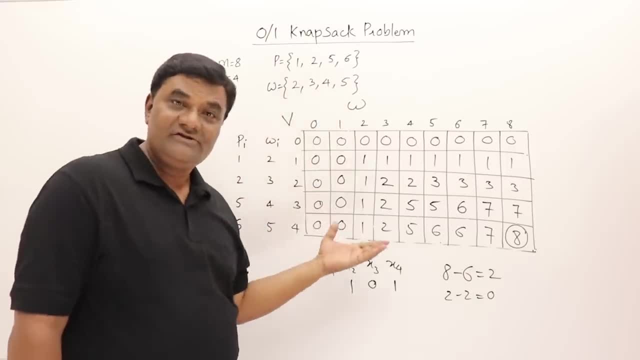 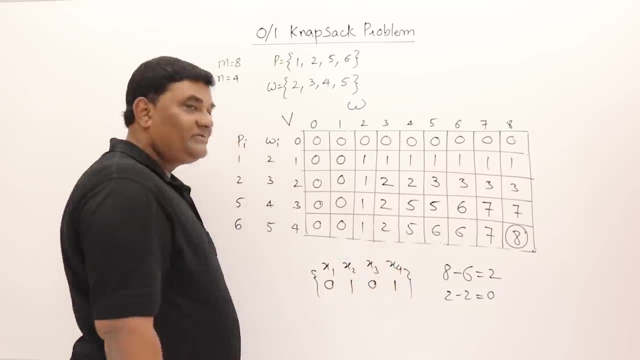 row. was it there in the zeroth also? yes, it was there in the zeroth also, this row also. so it means: don't include the object. so this is the solution. so it means which objects are anywhere in the back: x2 and x4. two objects are. 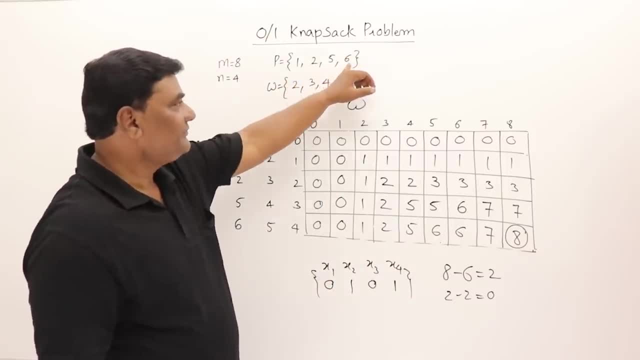 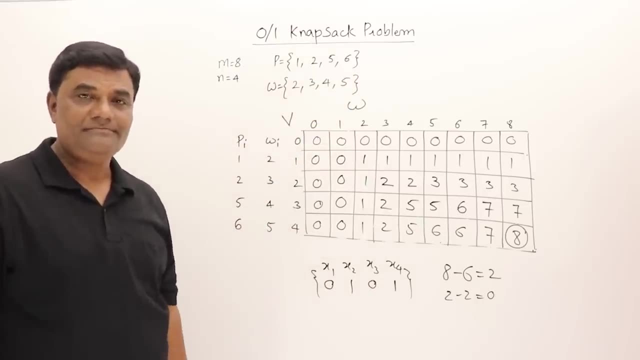 included in the back. so that is x2- is this one? x4 is this one. so total profit will be 8. so this is the maximum profit of 0. on knapsack problem next, I will solve it using sets method. same problem: I will solve it using set method. now let 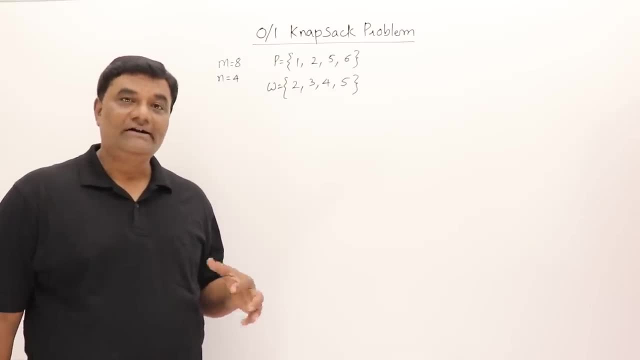 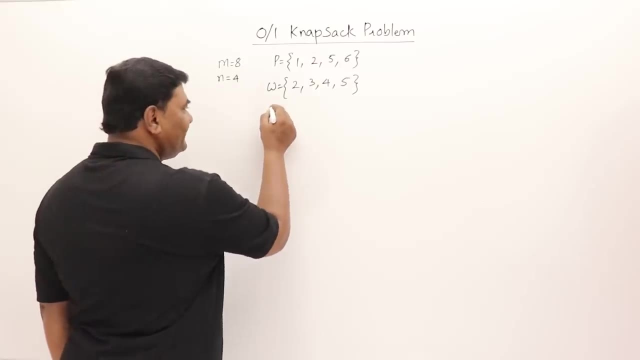 us solve it using set method. set method will try to find all possibilities and pick up the best solution. so let us see how sets are generated. we will prepare a set of order pair, that is profit and weight. so we'll start with the set: 0 set. 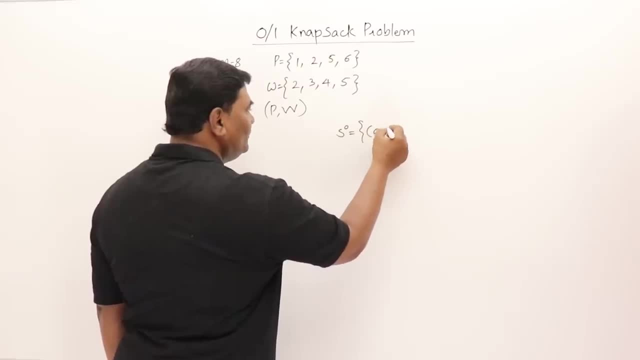 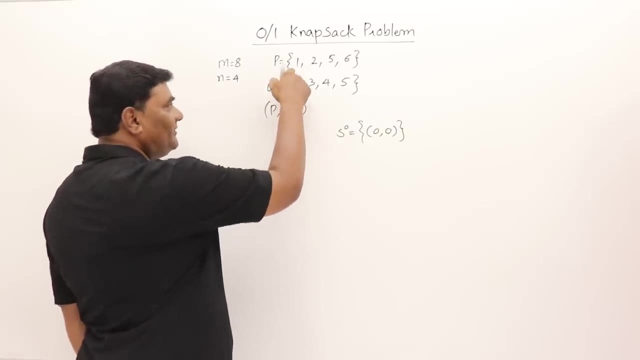 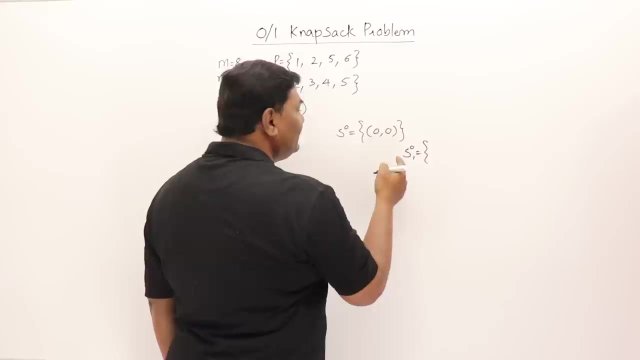 0. in this we say no profit, no weight means nothing is included in the bag. then we will consider the first object, that is, 1 comma 2, whose profit is 1 and the weight is 2. so consider the first object, so prepare s 0 of 1 and include. 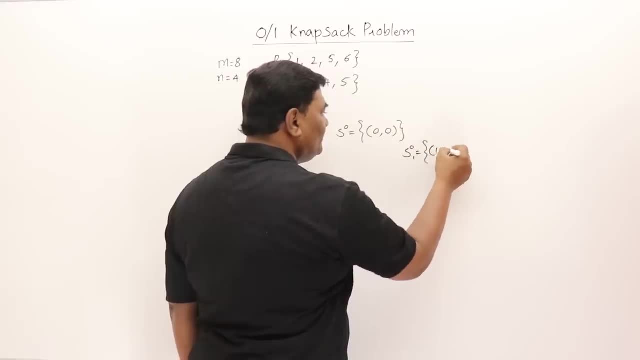 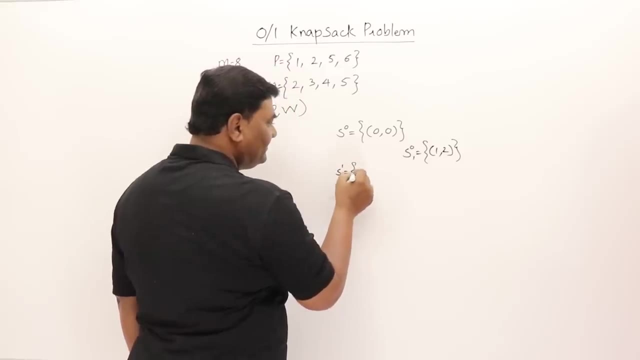 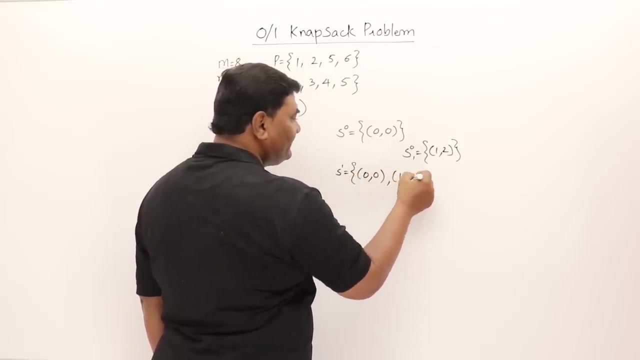 this first object in the bag. so it will be 1 comma 2. so actually add 1 comma to this order pair. so we get this one now, prepare set 1, then merge these two order pairs and prepare this one. so this means that we have considered first object. so two order pairs are showing that first. 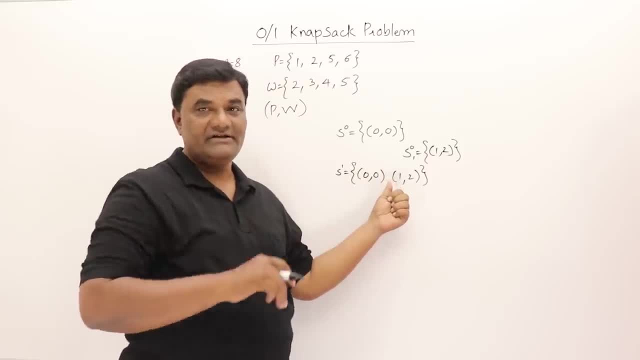 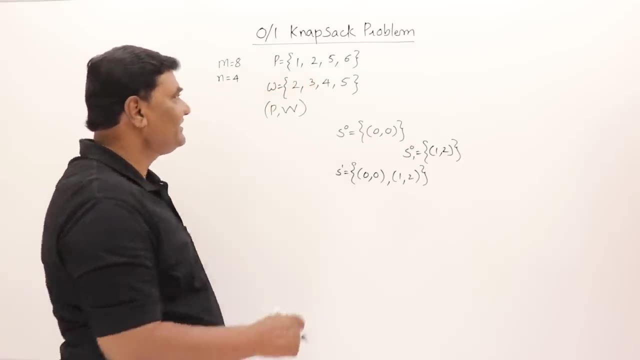 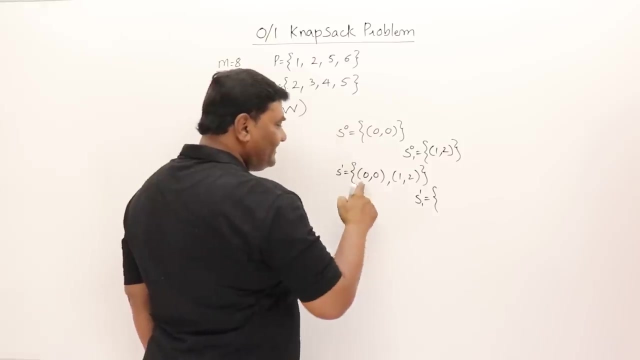 object is not included. first object is included. now let us prepare next set by considering second object, so that is 2 plus three. so prepare next set. that is s: 1, 1. so add 2, 3 to these order pairs, two plus 3, so this is two comma three. then 2 plus 3 is added, so this will: 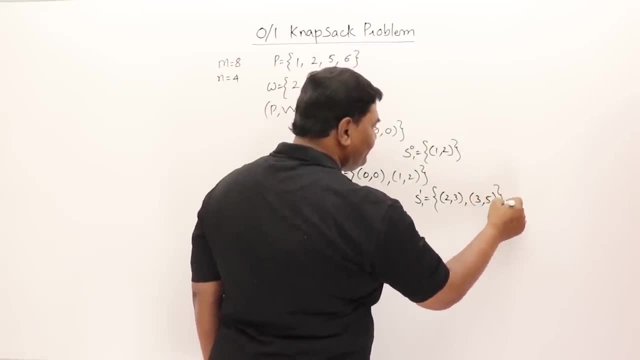 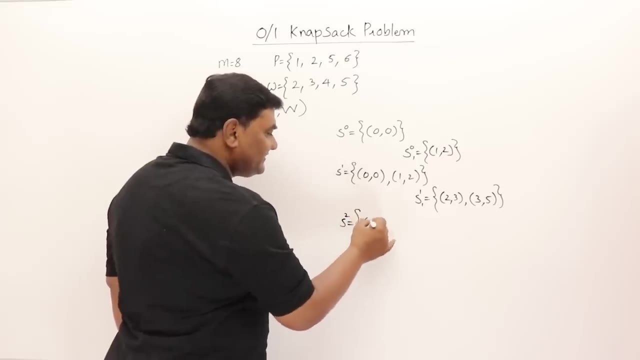 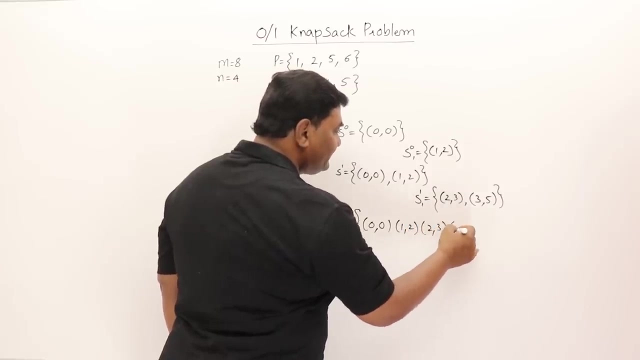 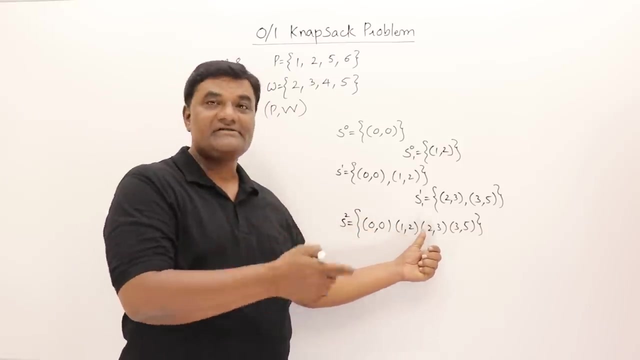 become 3 plus 3 comma 5, then this is second set for the second object. so when you consider second object, total four order pairs. all these are merged. so this is one, two and two, three. this is 3, 5. This means that no object is included. First object is included Second. 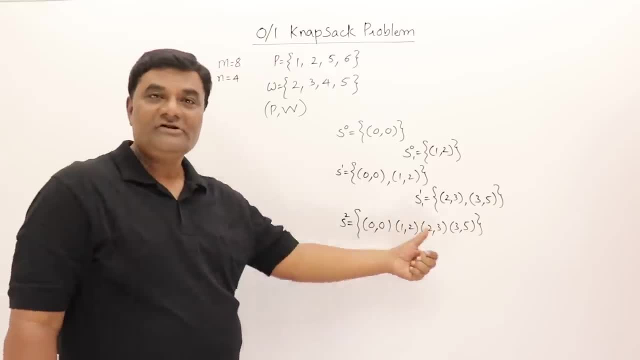 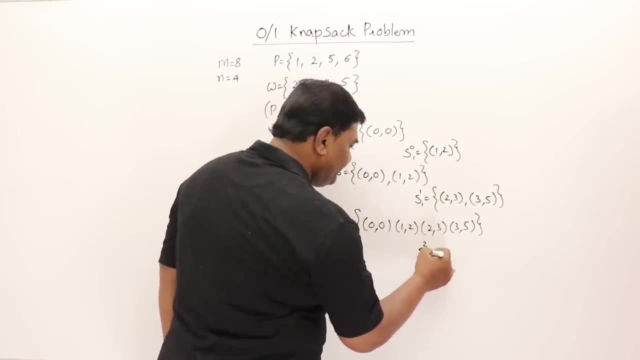 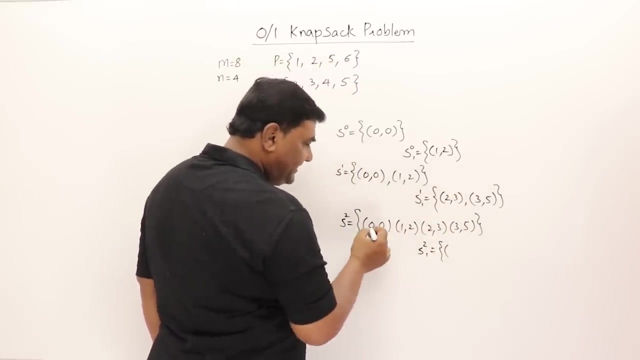 object is included. Both objects are included. Four possibilities are there, So all the ordered pairs we got. Then prepare S2 of 1 by considering third object 5, 4.. Add 5, 4 to all, So this is 5 plus 4.. So this is 5 plus 4. is 5 comma 4 only, So 5 plus 4.. So this will become 6. 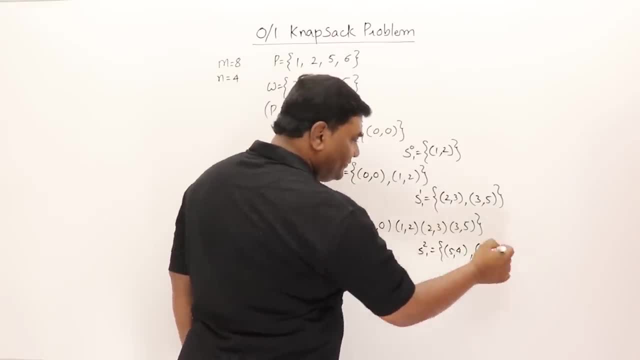 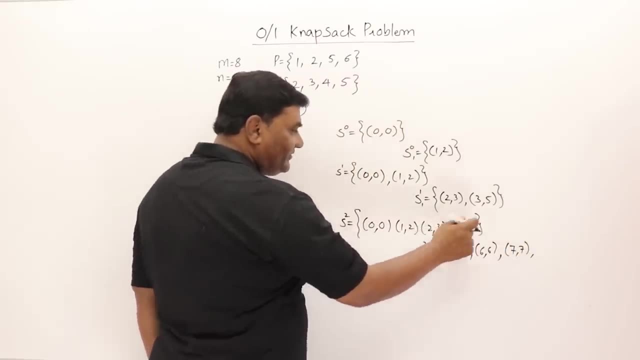 and 6.. So this is 6 comma 6.. 5 plus 4.. So this is 7 comma 7.. So 5 is added to this and 4 is added to this. So this become 8 comma 9, 8 comma 9.. Now merge all these and take: 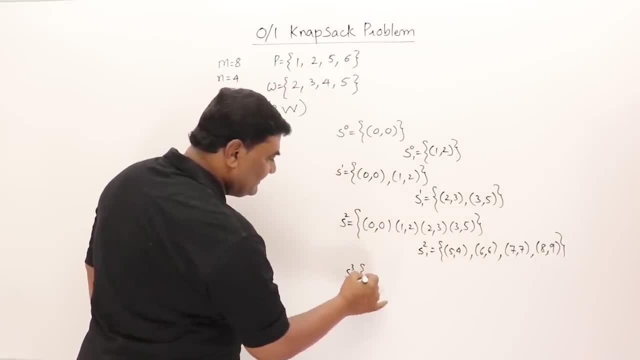 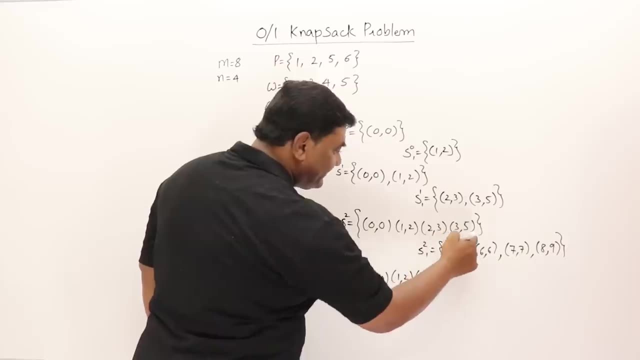 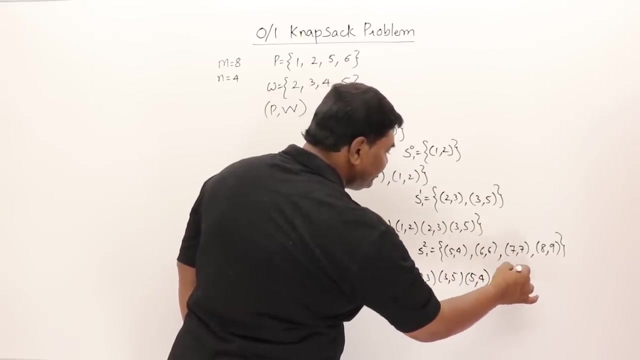 ordered pairs. So set 3, we get as 0,, 0,, 1,, 2, then 2,, 3, then 3,, 5,, then 5,, 4,, then 6,, 6,, 7,, 7.. Now here 8 comma 9.. Profit. 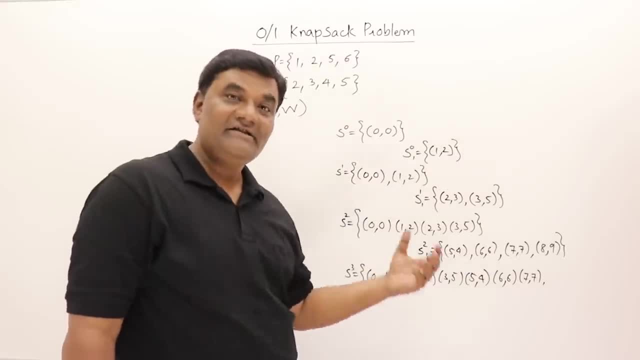 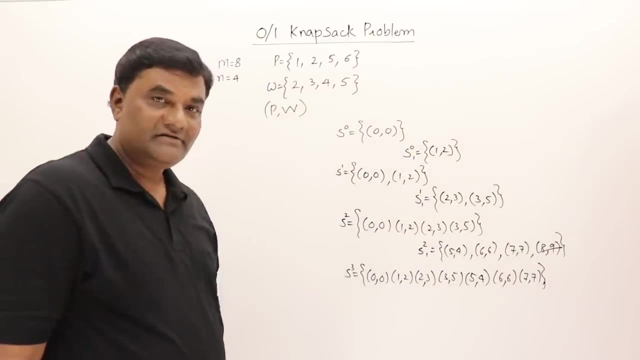 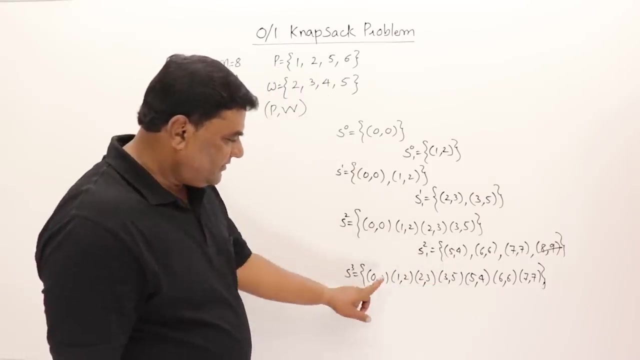 is 8 and the weight is 9.. So that is exceeding the capacity of the bag. Don't include that one. So we have discarded. Now this is set 3.. In this one, if you observe, this is profit. this is weight Profit increased. 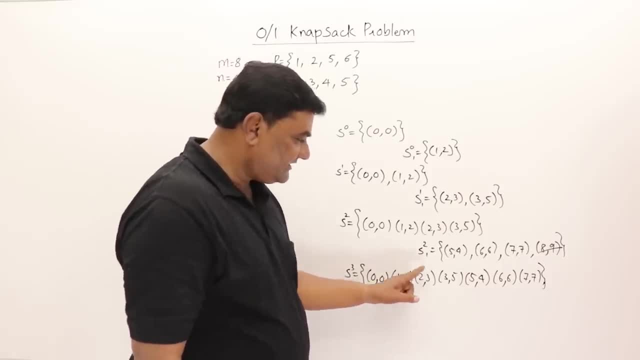 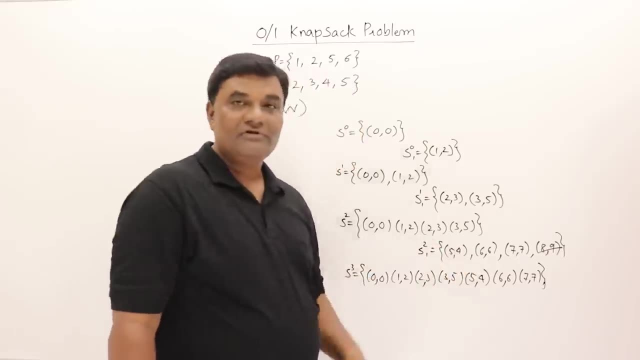 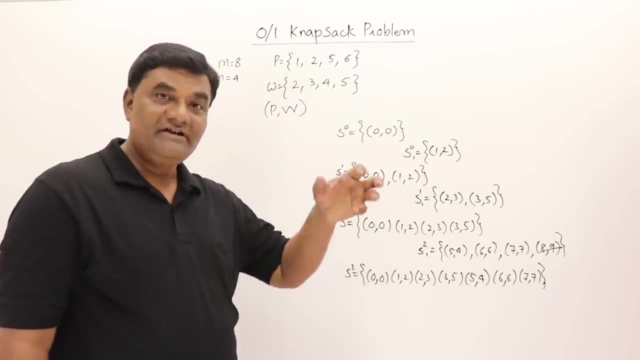 weight increased. Then from this profit increased, weight also increased, Profit increased and the weight also increased. But here profit increased, weight is decreased from 5 to 4. This is not possible. Profit is increasing, so the weight is also increasing, But weight. 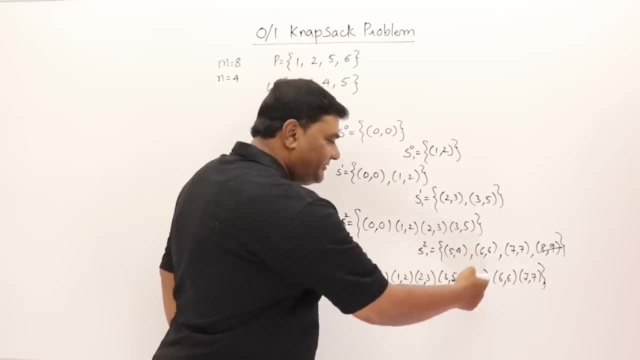 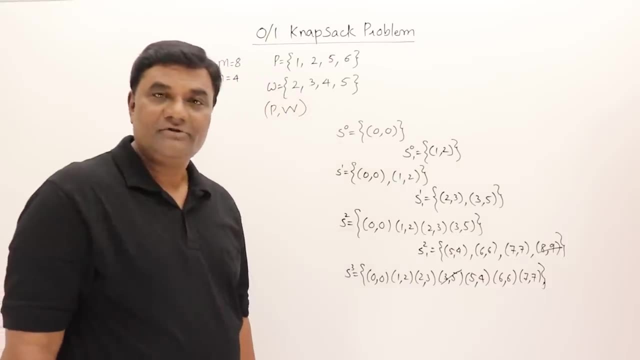 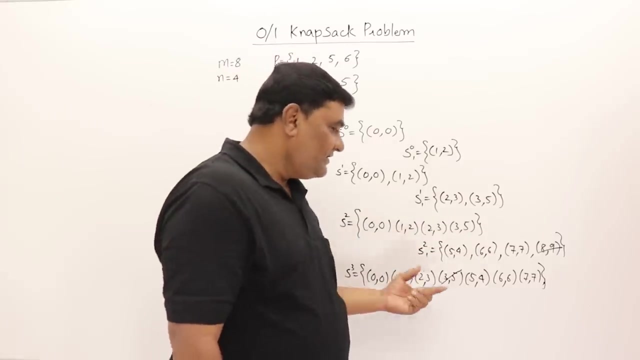 is decreased. How is this possible? So that is why this order pair are wrong. So we have to discard any one. So we will discard the one with the lesser profit, smaller profit. So 1,, 2,, 3,, 4,, 5, 6.. Now we have only 6 order pairs because 2 were invalid. 1 was. this was: 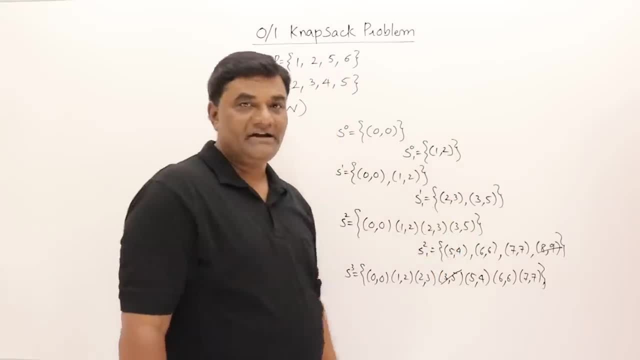 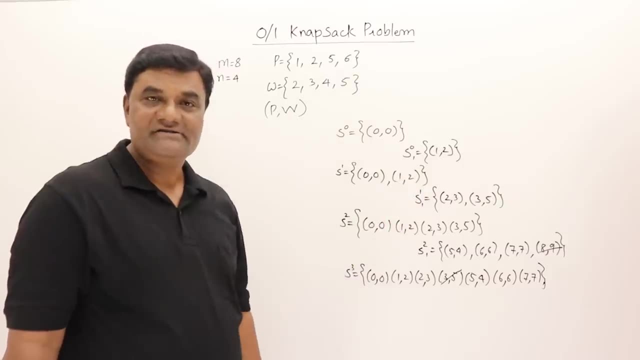 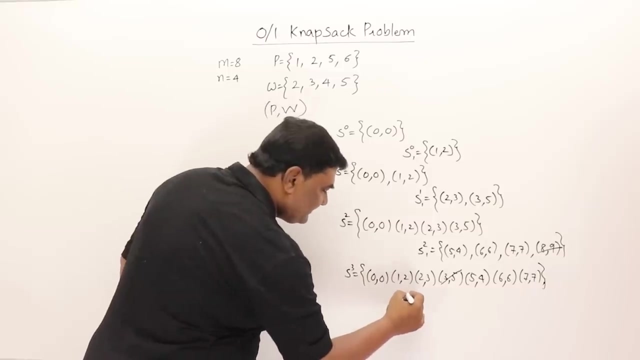 giving wrong values and this was exceeding the capacity of the bag. So cutting off this one, we call it as a dominance rule. So with the dominance rule the value is order pair is discarded. Now I will consider fourth object 6 comma 5. I will include. so I will prepare set 3: 1 by considering: 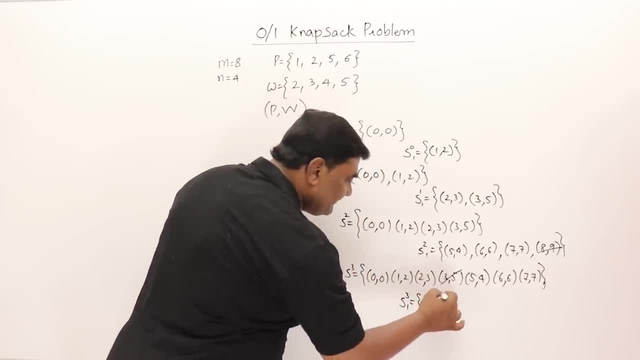 fourth object: 6 comma 5. so first order pair is 6 comma 5. next order pair is 6 and 5 are added. so this is 7 comma 7, then 6 and 5 are added, so this is 8 comma 8 and then 6 and 5 when they are. 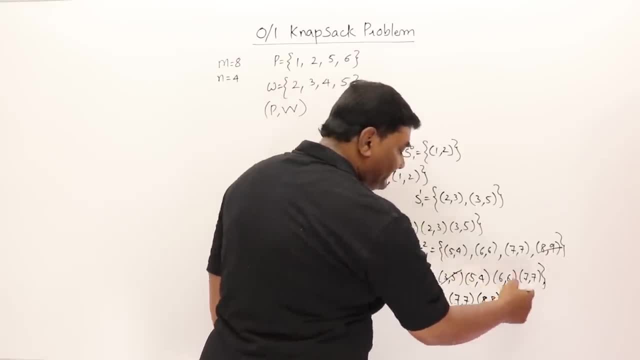 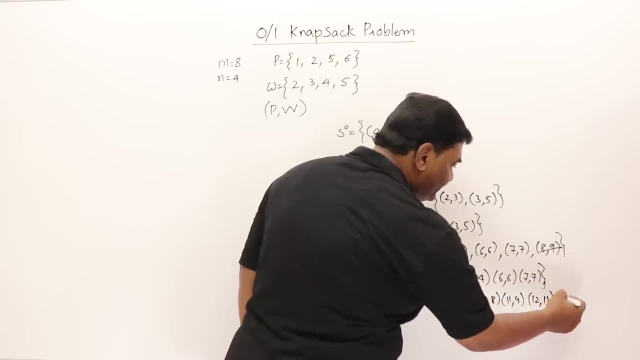 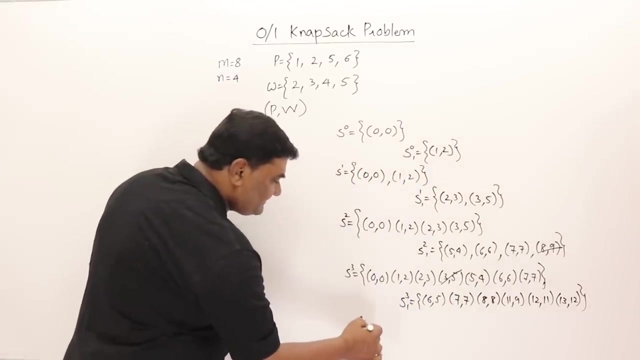 added, it will become 11 comma 9. 6 and 5 are added, so this become 12 comma 11 and 6: 5 when added to 7 and 7, so this becomes 13 comma 12. now I have to prepare set 4. this is the final set. 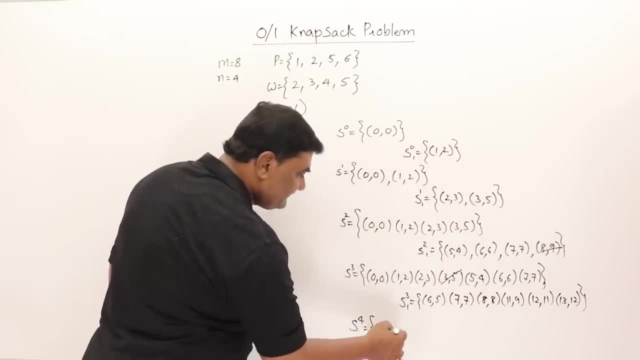 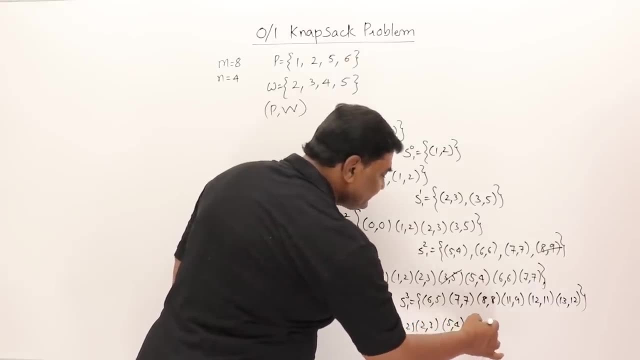 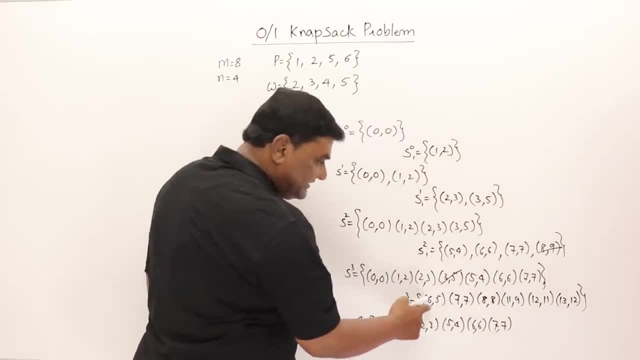 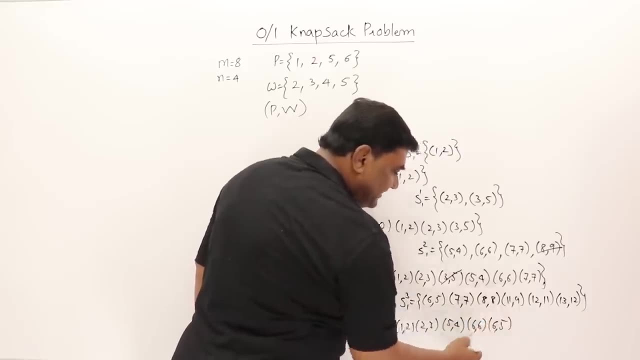 7 comma 7. they are coming. as it is now in this one, 6 comma 5 is there. so 6 comma 5 should come before 7 comma 7. so 6 comma 5. now, here again, you see, the profit is remaining same, but the weight. 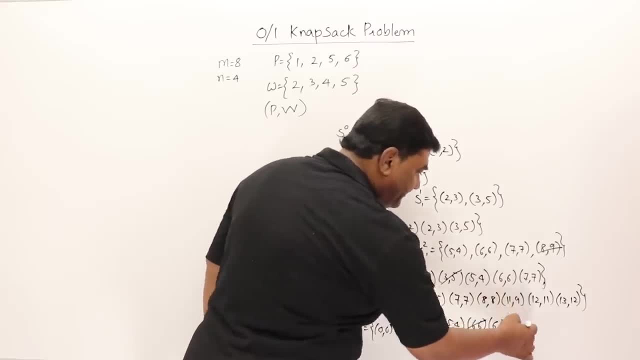 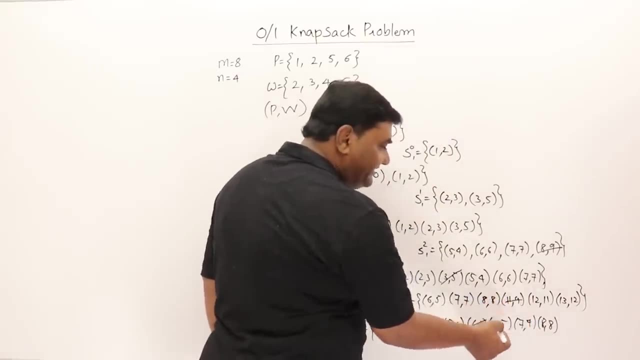 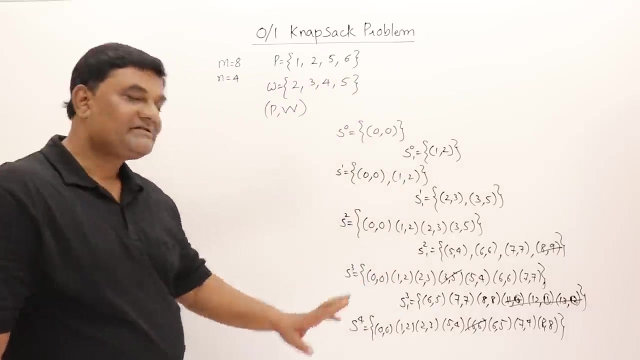 is reducing, so this should be removed. then 7 comma 7, is there. then 8 comma 8, is there then remaining 11 comma 9, exceeding the capacity of the back? 9, 11 and 12? so all three order pairs are gone. so these are the order pairs I have. so, if you observe, the method is generating all possibilities. 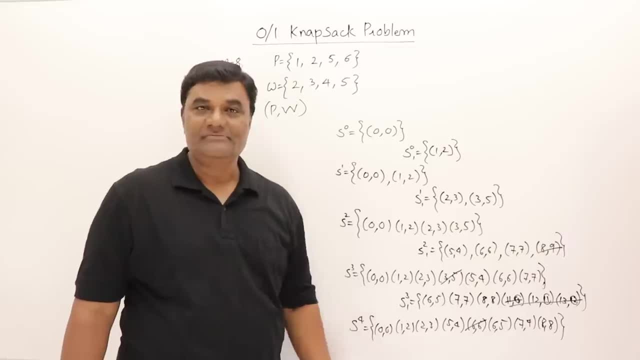 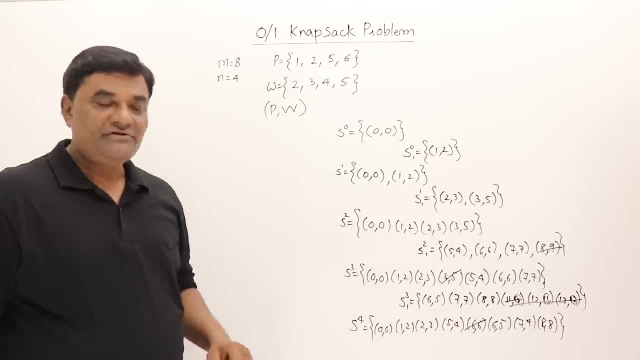 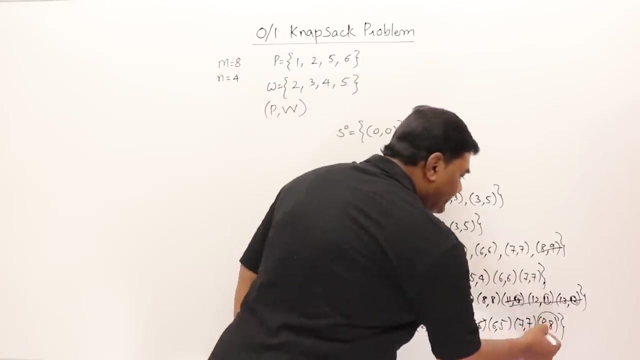 so this is one easy method of finding all possibilities. so the time taken by this one is almost 2 power n. now what is the solution? so we have already sets, now we take the sequence of decisions to solve this one. now what is the maximum order? fair, 8 comma 8. so 8 comma 8. 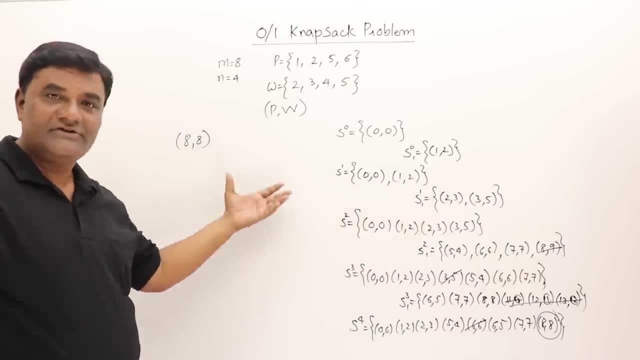 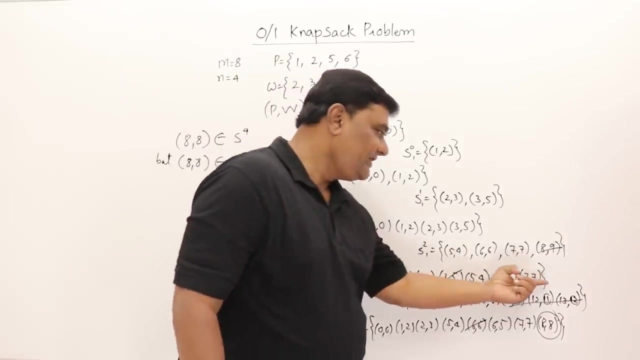 using that I will solve this one. so the approach is similar like what we saw in the tabular method. 8 comma 8 belongs to set 4, but 8 comma 8. check whether it belongs to set 3 in the set 3 8 comma. 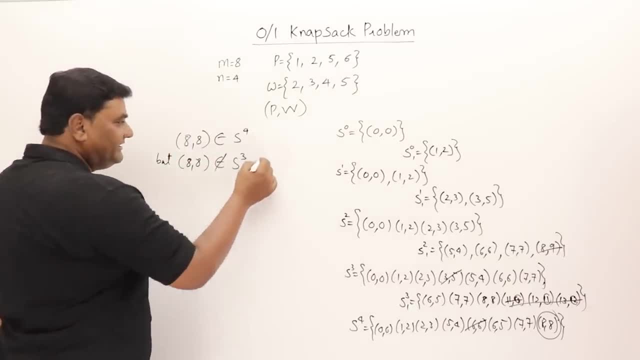 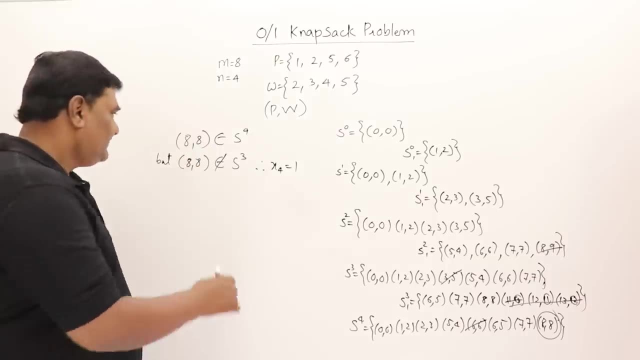 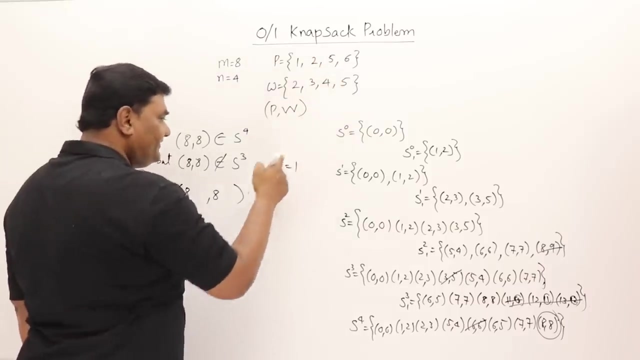 8 was not there, so it doesn't belong to set 3. therefore fourth object is included. because of that only, we got 4 comma 4. now I should take an order pair 8 comma 8. from this I should subtract the profit and weight of the fourth object. so this is profit. 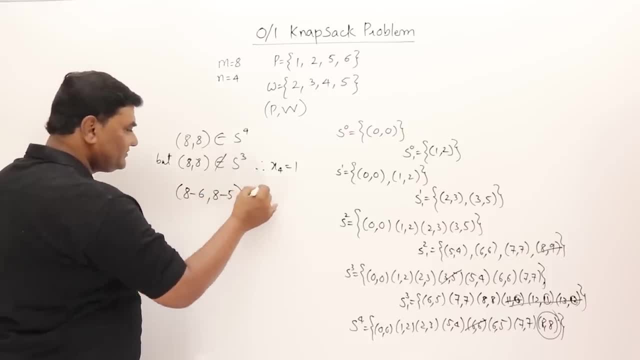 is 6 and the weight is a 5, so the order pair is: how much? 2 comma 3. so now I should consider 2 comma 3. so now, this was the first one. now second one: 2 comma 3. now I have to consider third object. 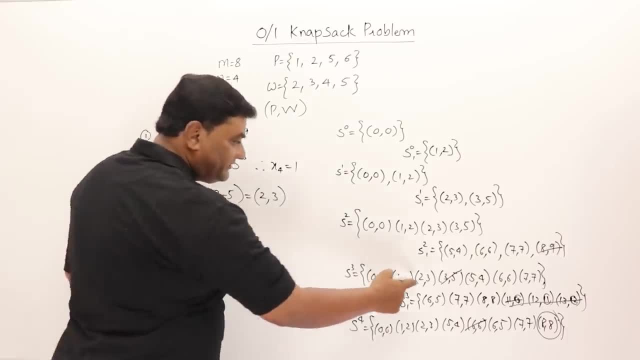 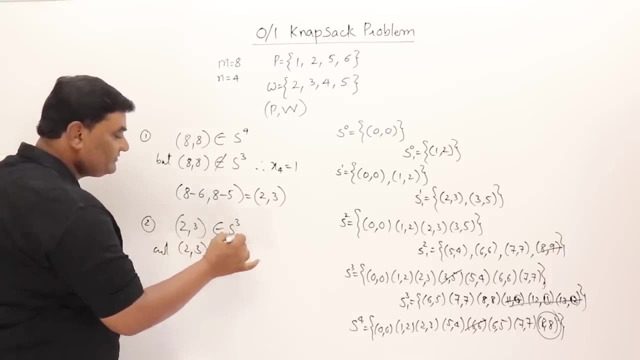 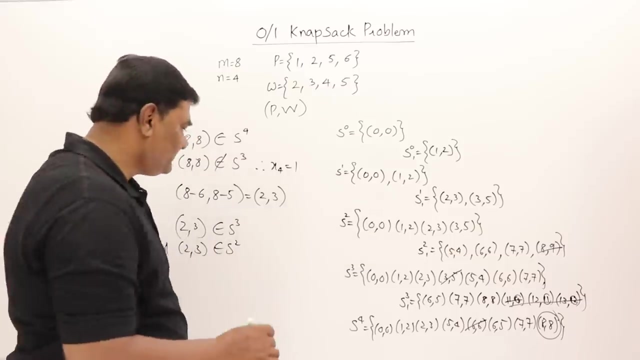 so check whether it belongs to s3. 2 comma 3: yes, it belongs to s3. and 2 comma 3 belongs to s2. check whether it belongs to s2. yes, 2 comma 3 is there here also. it means this is not because of the third object. so therefore third object is not included in the 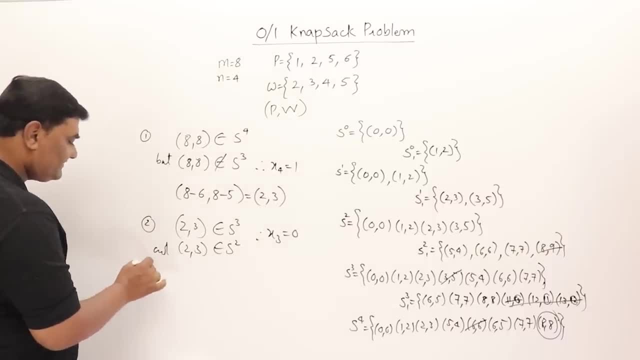 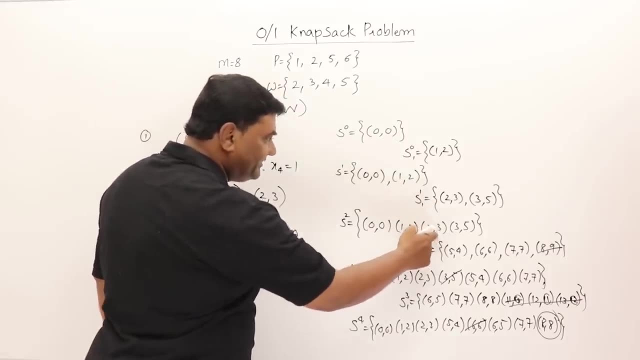 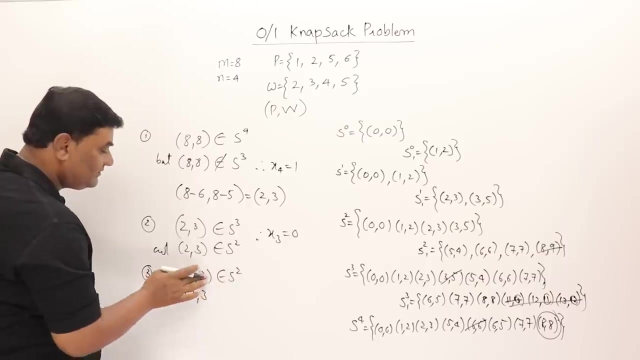 back then. now next step is I will consider second object. 2 comma 3 belongs to set 2. for second object 2 comma 3 doesn't belong to set one, so 2 comma 3 was belonging to set 2 and and 2 comma 3. 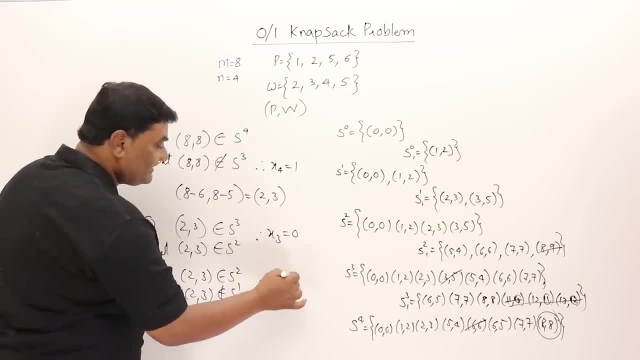 doesn't belong to set 1. so therefore this is because of the second object included. now what is the profit and the weight of the second object? 2 comma 3. so when you subtract 2 comma 3 from this one, 2 minus 2 is a 0 and 3 minus 3 is 0. so this gives 0 comma 0. now i should check the right answer. 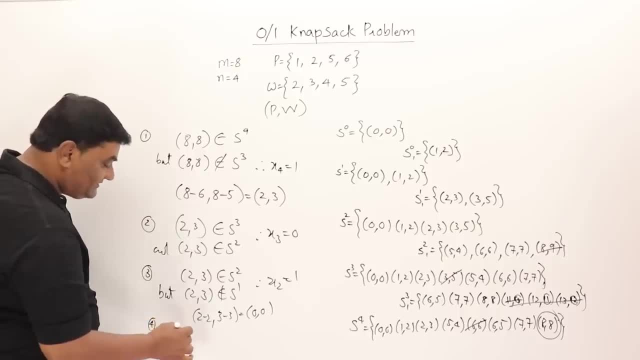 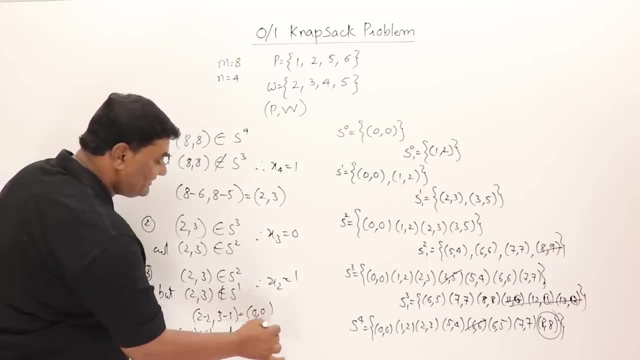 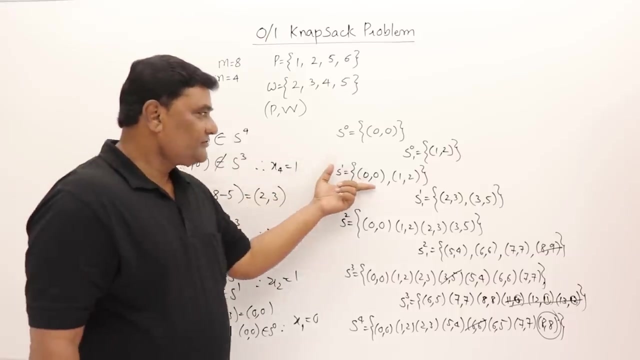 I will consider now. the step is 4, so 0 comma 0 belongs to set 1, and also 0 comma 0 belongs to set 0. therefore first object is also not included. 0 comma 0 belongs to s1, also s0 also. it means this is obtained not because of the first object. 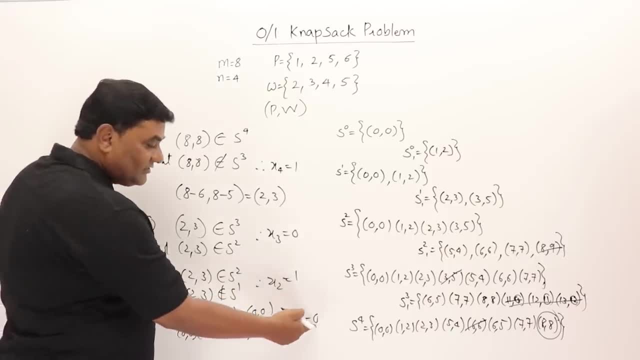 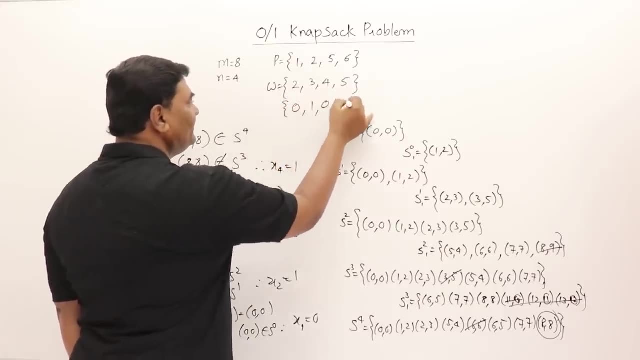 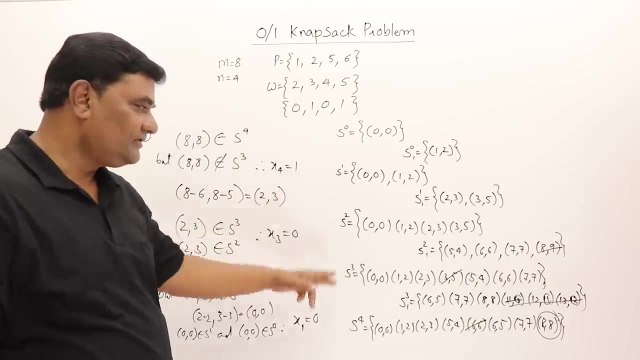 So first object is also not included. then the solution is from bottom, if you see 0 1 0, 1.. So the answer is 0 1 0 1. so these two objects are included. see, the profit is 8. So we got a same solution with the help of sets also. So this is one more method.